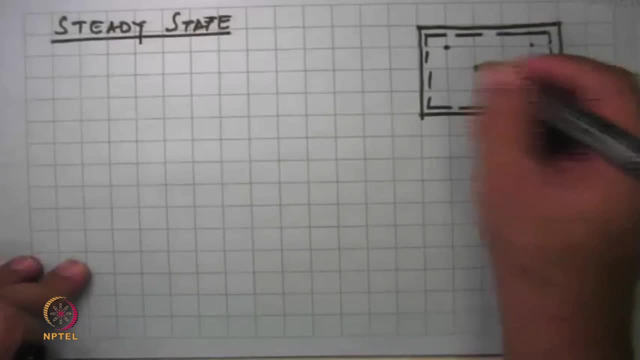 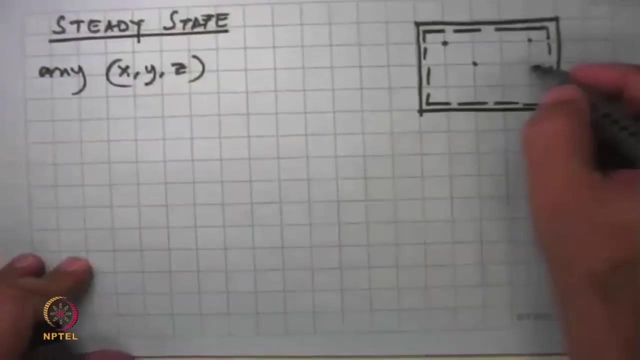 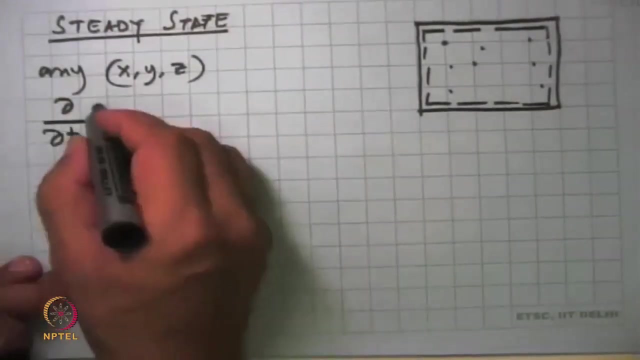 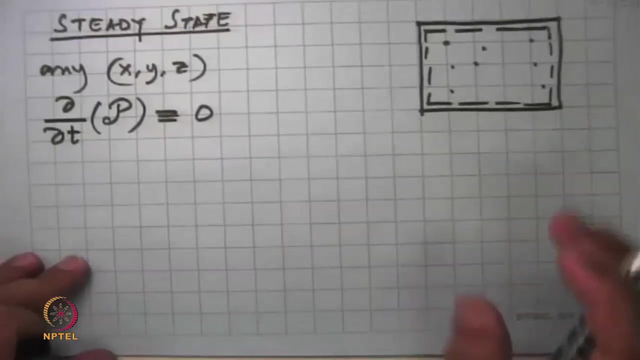 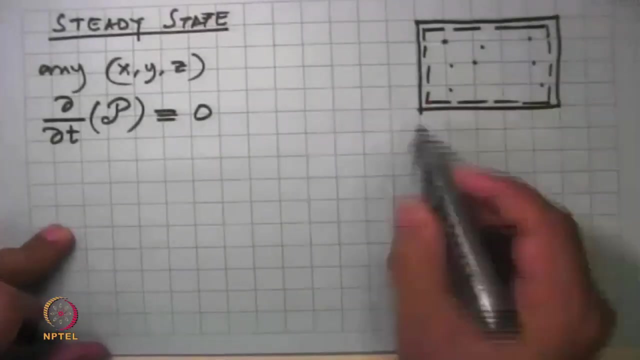 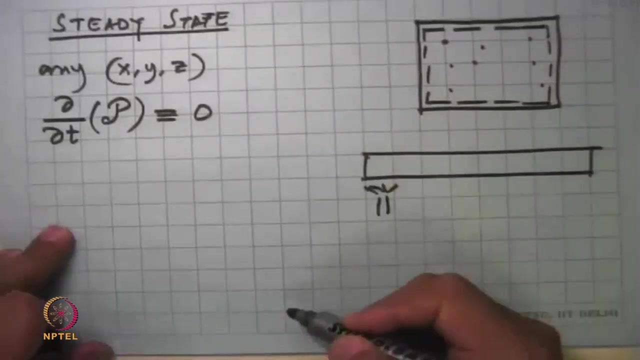 Then at: if at any point- At any point Means any physical location at any point in the system- there is no change of any property with time, any property, then the system is in steady state. ok, So what we are saying is that if I have a rod and I am hitting it at this end and allowing it to cool, like 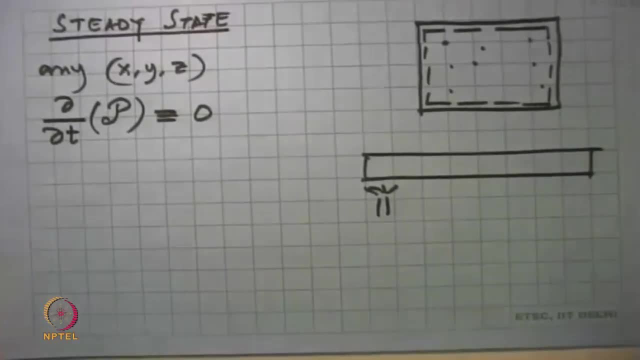 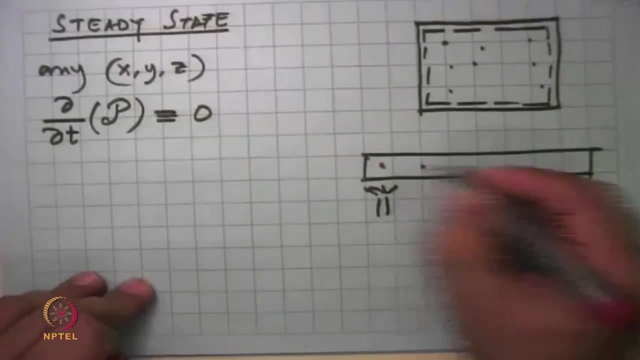 that the other end And let this system be operating for a very long time, then what we know is that the temperature at the core here is higher and it is decreasing as we go up. So the temperature is a function of space. 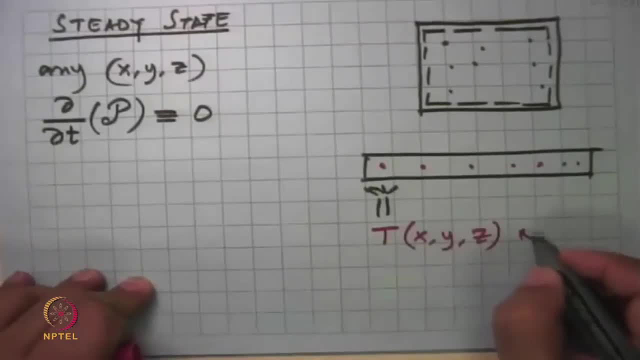 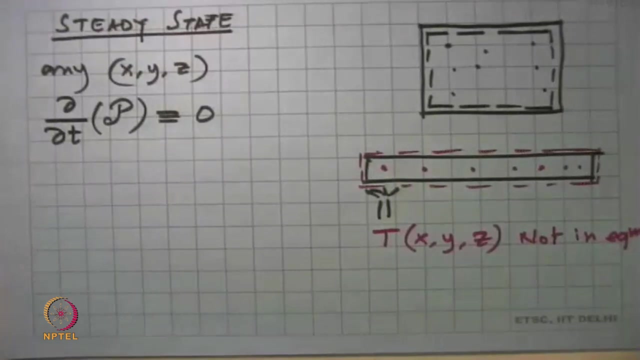 So it is just a value. So at any point It will be. the system is a system of space. So, if you remember we have, what we are saying is that in the system it is not, And so this rod is. if this rod is taken as in system, this rod is not in equilibrium. 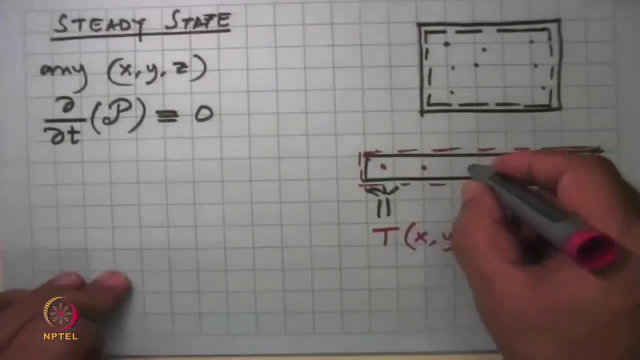 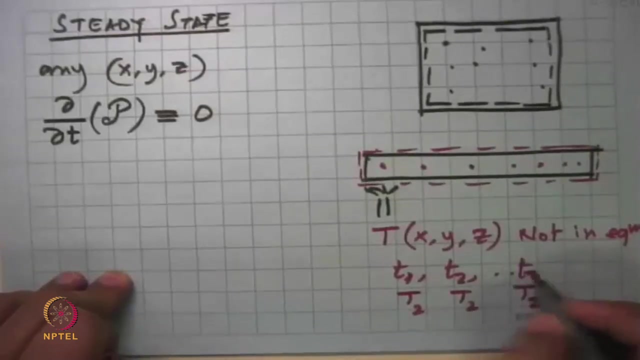 but if I stand here and I keep measuring this temperature now and after 5 minutes and after 10 minutes and like that, and if at any instant of time, T 1, T 2, like that, the temperature is still the same, say whatever it was, T 2, T 2, T 2 at any instant of time, then the system 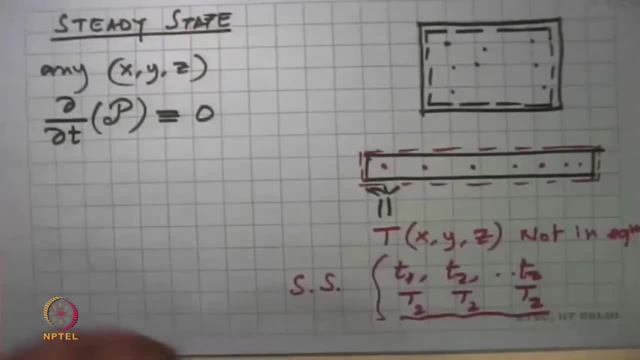 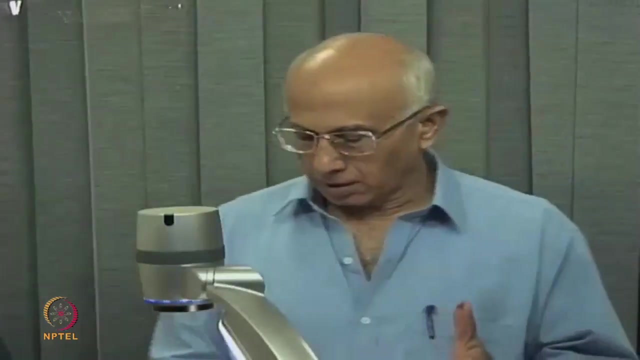 is in steady state. This simple definition has very far reaching implications. the most obvious- something we talked yesterday- a lot about solar, solar energy falling on any collector- photovoltaics or any type of a thing- is always changing with time, And so this is what we are talking about. 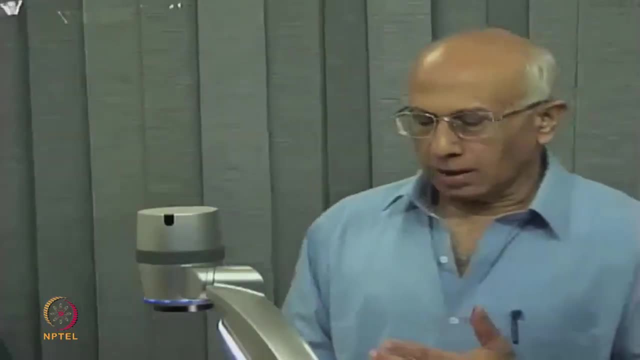 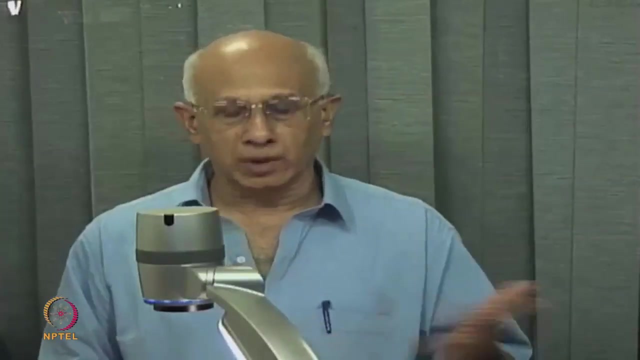 and from sunrise to sunset it undergoes a value. after that it becomes 0. So that is the biggest problem is solar energy. it is not steady In a nuclear reactor. we can manage it so that the heat generation in nuclear reactor is steady, steady with time and then. 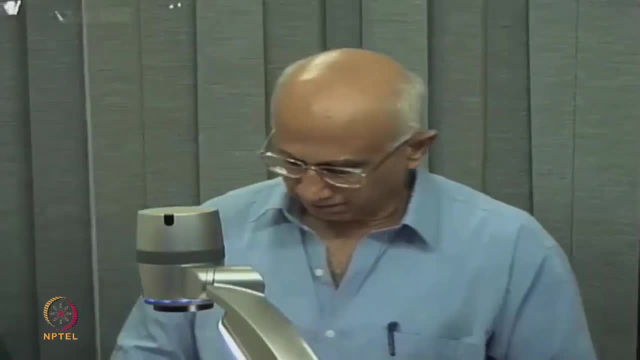 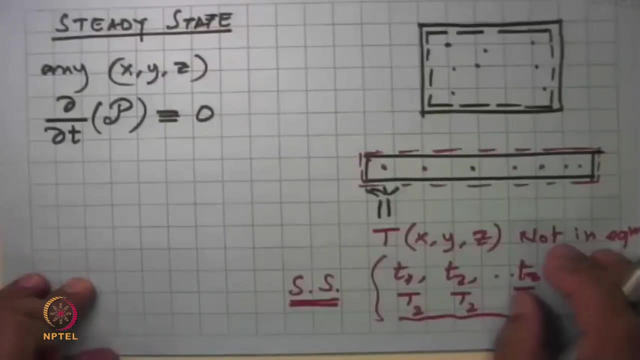 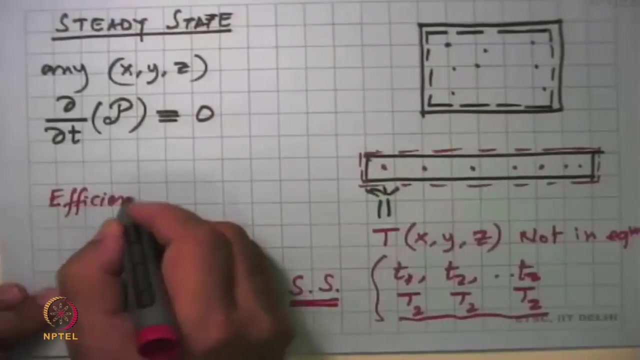 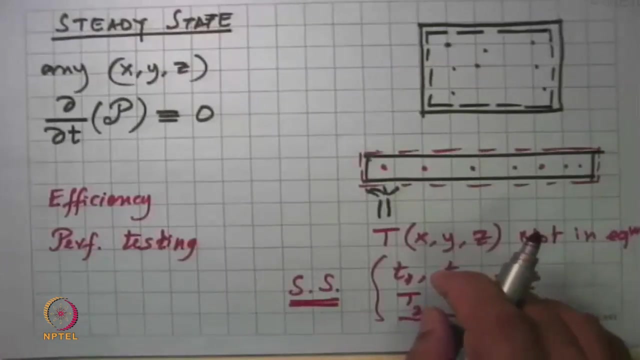 you can get continuously a constant generation from the system. So that is an example, but this has got lot more things to do with it When we will talk later on and we talk about efficiency or performance testing, all these analysis, whether it is for standardization- 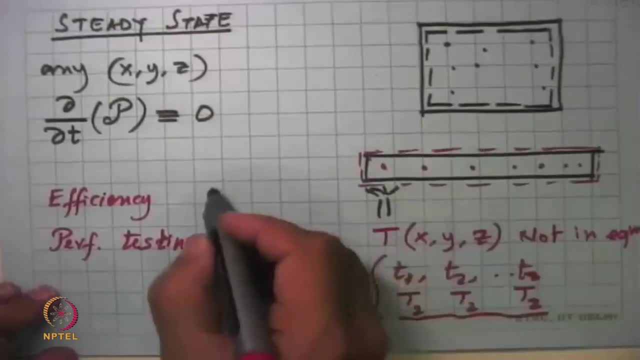 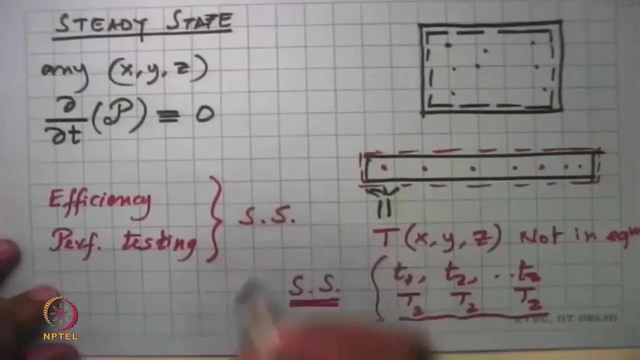 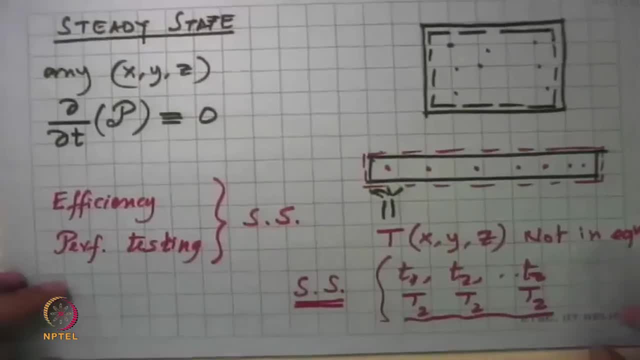 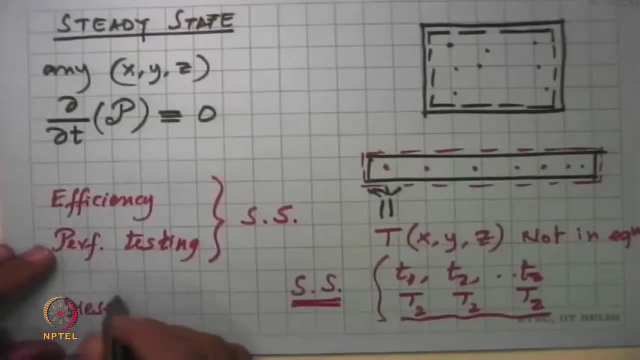 time, the industrial systems are not in steady state. So, for example, if you want to test a diesel engine and say what is the kilometres per litre a car powered by diesel engine, or say a bus and say what is the kilometres per litre that I get, then the right thing. 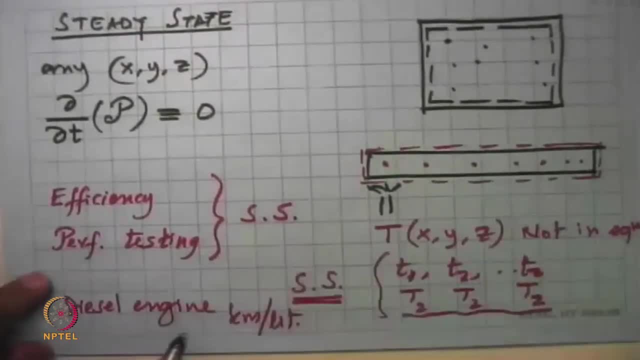 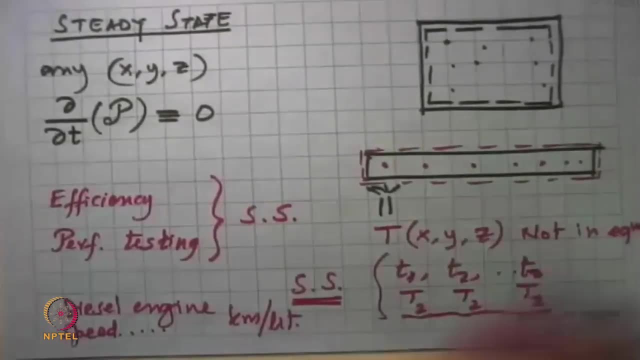 to do would be say: well, look, which gear will I drive, what speed will I drive? all of that is specified. what is the condition of the road, what is the ambient air temperature and pressure, which fuel we are using, what is the health of the engine? all these things. 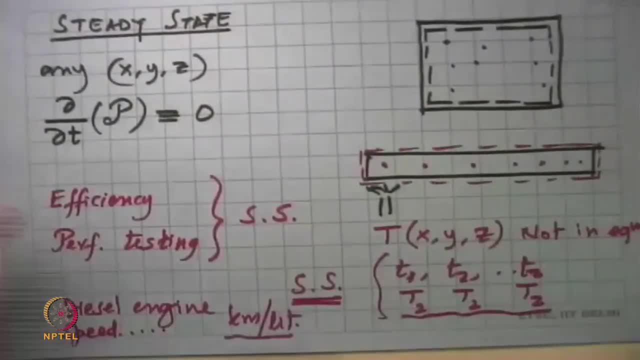 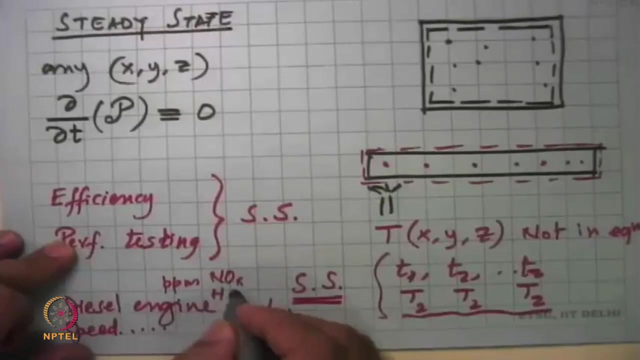 have to be first well controlled, And then we operate it at a constant load for certain period of time and then say: this is the fuel economy of this, or how many? how much ppm of NOx does it throw out? or how much hydrocarbon does it throw out? or how much particulate? 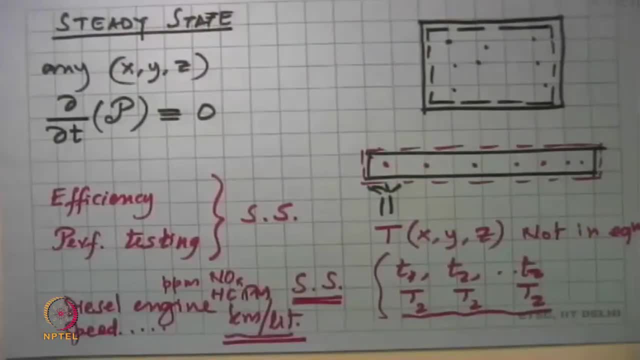 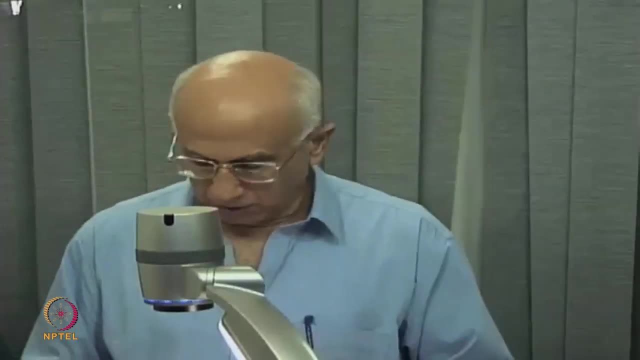 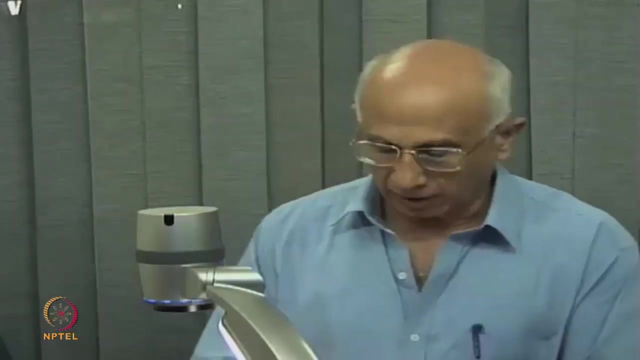 matter. does it throw out? that is what one would do with a diesel engine. Look at the real life. anybody who has been in traffic in cities like what we have heard, all the mess that we saw in Gurgaon or in Bengaluru and recently in Delhi of the rains, even if those were not there in normal times- 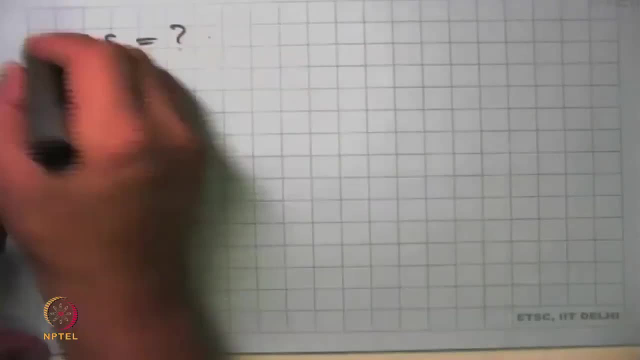 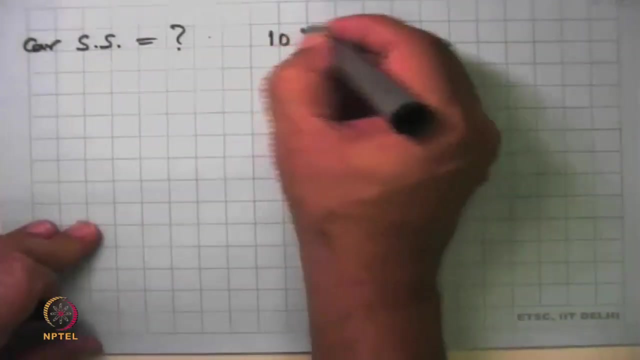 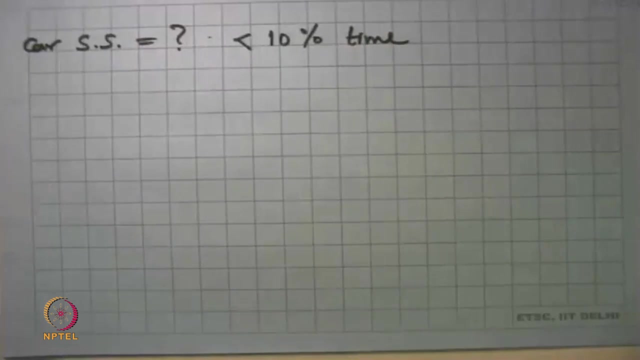 do we have steady state driving in a car? We made a measurement and we find that steady state operation is restricted to less than 10 percent of the time that a vehicle moves on a road, in many cases even less on the highway. it is going to be more, it is slightly. 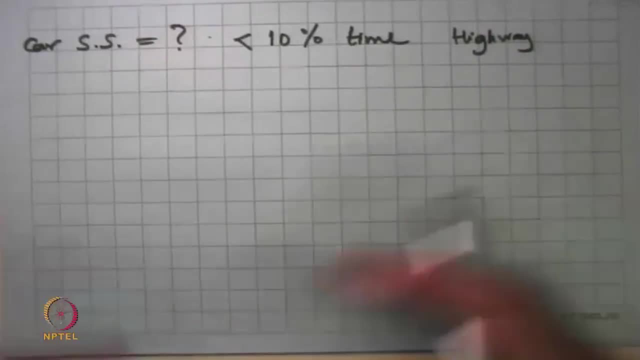 more than this, but not very large. If the highway is clear, no other traffic, the road is flat, everything is nice and clean, no winds, then ok. So in city conditions you never have steady state. So to say what is kilometres per litre of a car is basically. 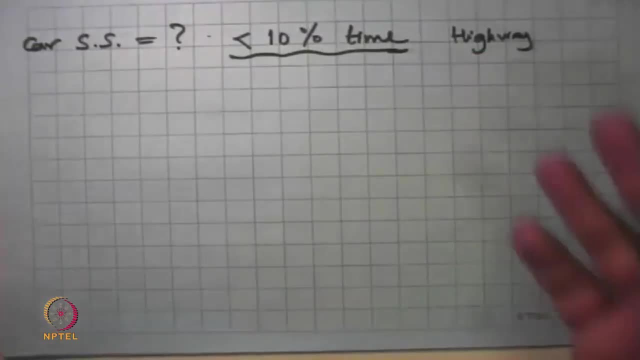 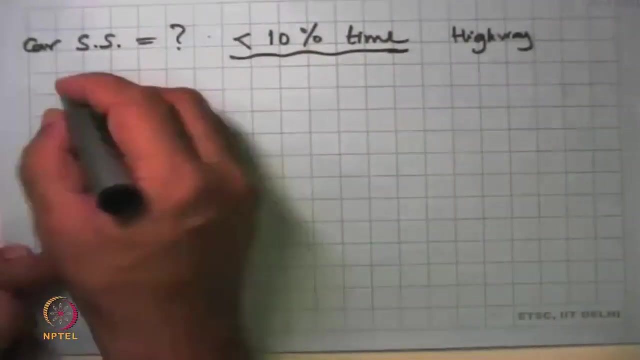 admitting that, look, I cannot be bothered whether it was steady state or not. how much did I get? that is the only thing I will talk about, and that is fine. Then, if you look at any of the power plants, whether it was nuclear or gas, whether it- 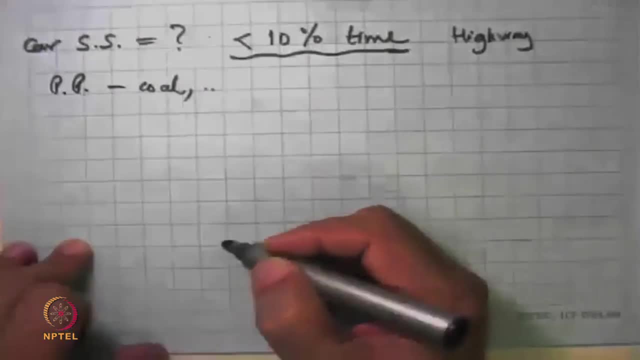 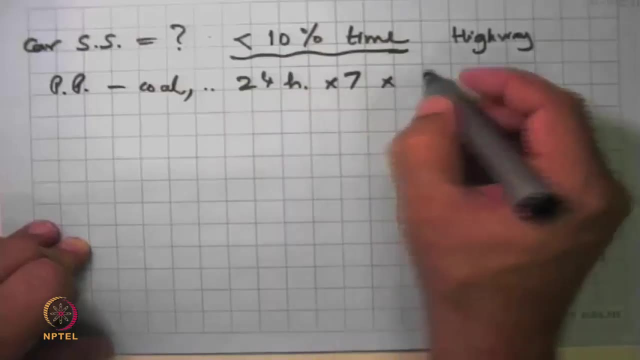 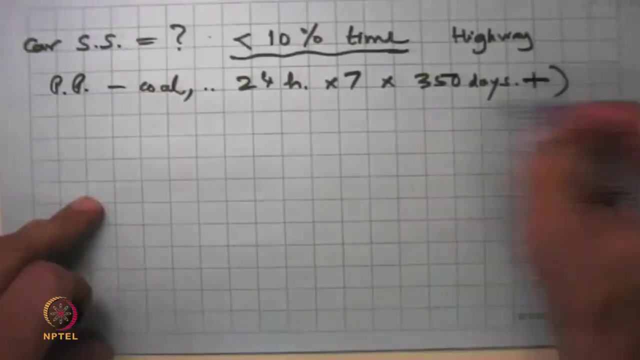 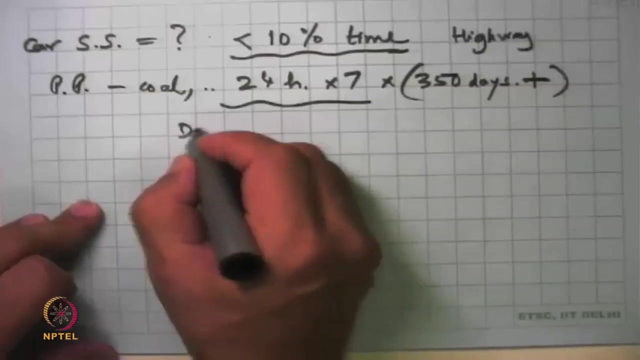 was coal or anyone. the plant is operating over 24 hours, 7 days a week, and typically it will run at least 350 days a year without stopping. may be even more these days, But what happens? During the day time, the demand for electricity is more. at night, almost all. activities are stopped, So the demand for electricity is more. at night, almost all activities goes down, the demand is less, and the electrical grid system is such that the generation has to always match consumption, So generation has to be exactly equal to consumption, which 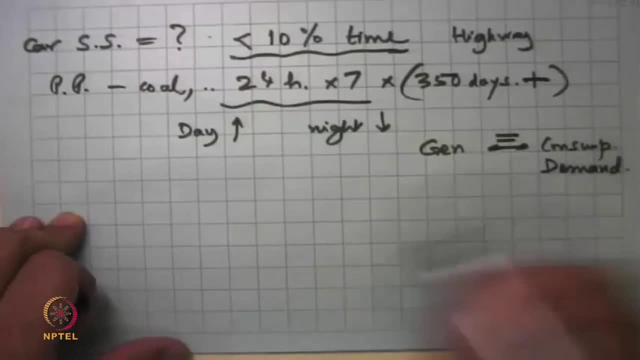 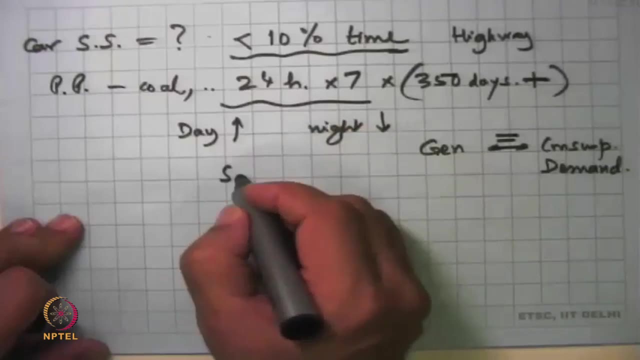 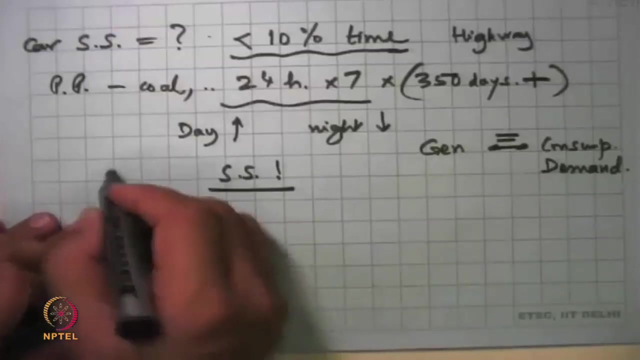 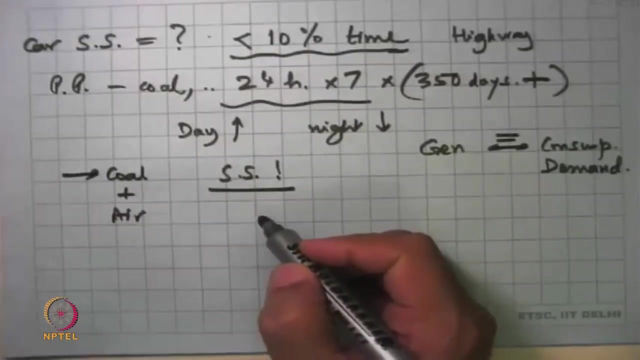 we are called demand, And when that happens, this power plant will never ever operate in a state. Another thing that will change the operation is that when you are burning, say, coal or oil with air, the coal has to be in steady state, all its properties must be same over 24 hours or more, And air also, all the properties must. 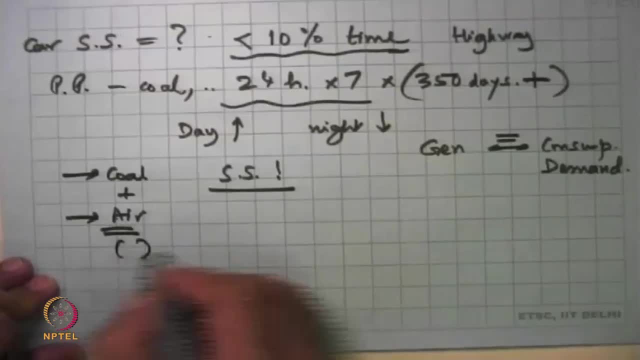 be same but, as you know, air undergoes a maximum temperature and a minimum temperature, and some humidity also. So dry bulb temperature goes up and down, the relative humidity goes up and down. So the temperature goes up and down, the relative humidity goes up and down. 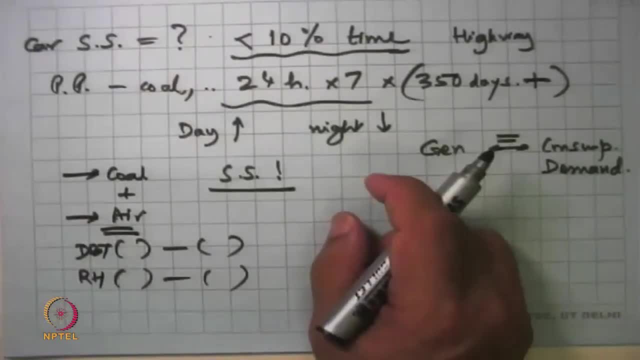 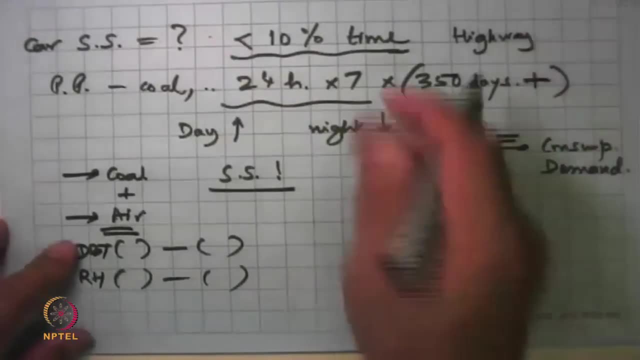 so the air going into the boiler is also not in steady state. The demand is not in steady state, So if I have to do an efficiency test or emission test on a power plant is extremely difficult, And so we have codes and standards which will give you the best possible way. 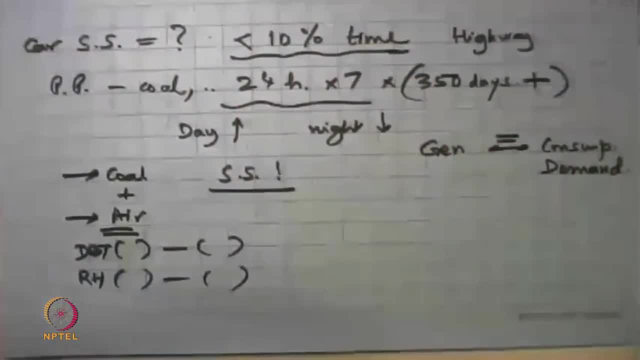 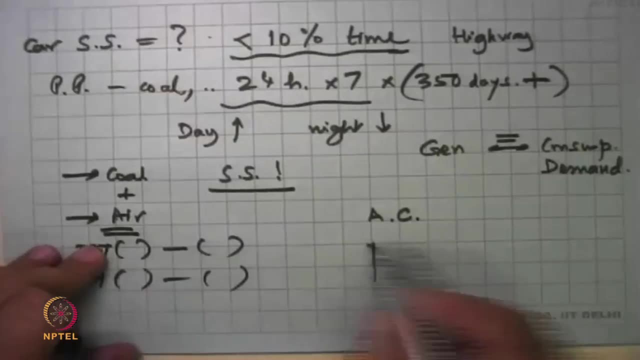 to measure it. But if a system can be well controlled, for example if you are doing the efficiency test of an air conditioner- then there is a well designed setup. where you have one. the AC is a window, AC is sitting there. One channel is there, another one is. 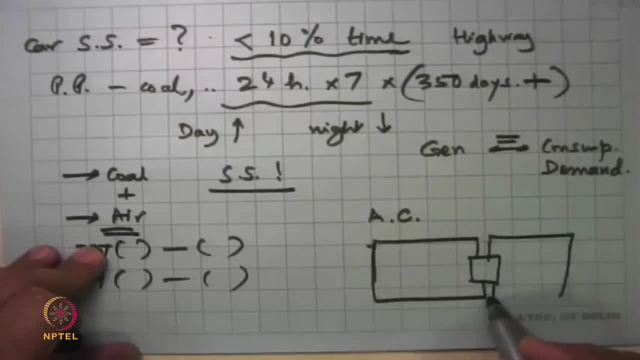 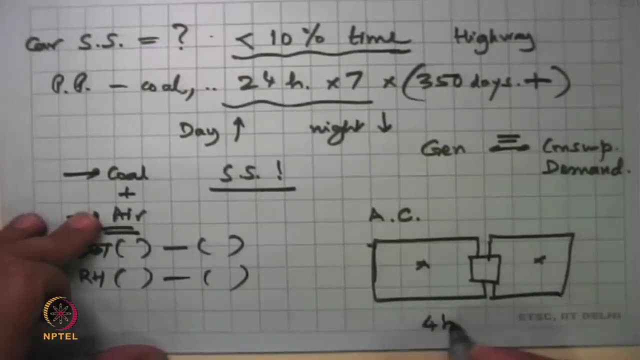 there, one chamber here which is the hot side, one chamber here where you cool it. We maintain the temperature of these two constant and make sure that the system is in steady state for at least 4 hours and then we take the reading, and this is completely isolated. 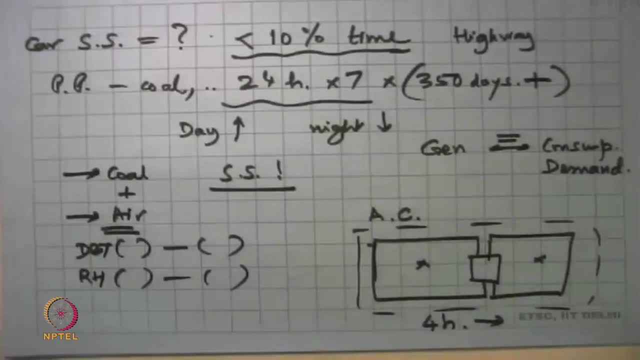 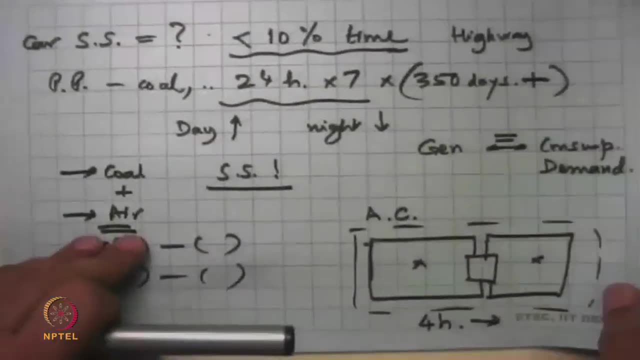 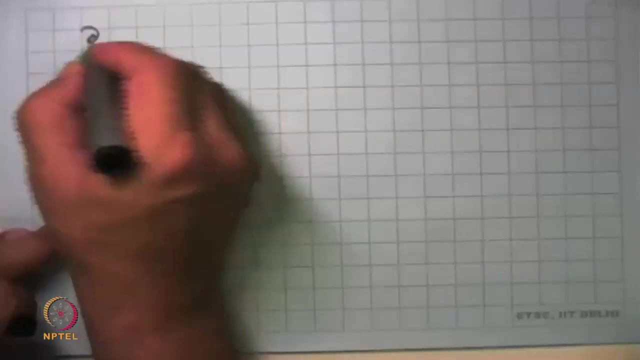 from the surface. Then you have a very, very reliable way of measuring its performance and then the efficiency makes sense. In reality, this may not be happening. So steady state is a very important component, but since many of these systems do not follow in steady state, we can say: well, is the time dependence of the property very small and 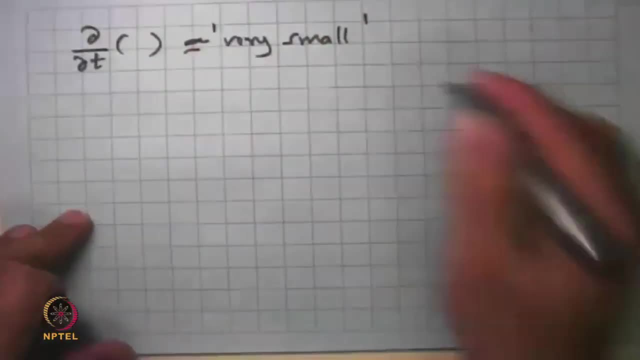 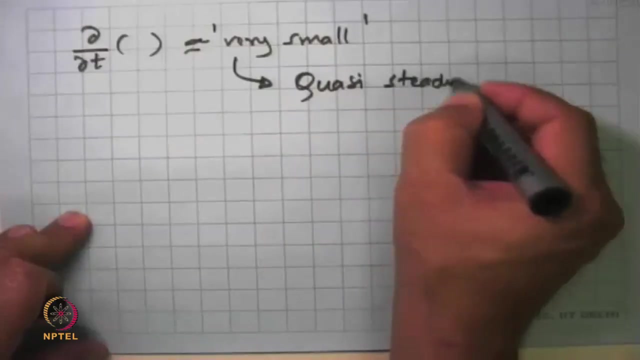 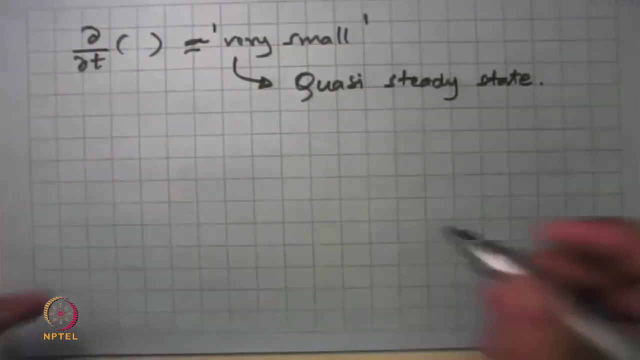 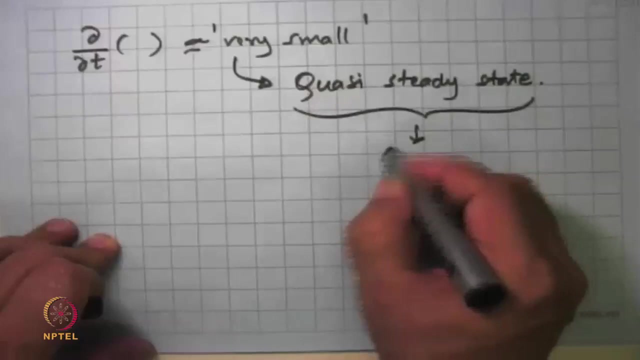 how small that our discretion, And it is a. it is small means ok, it is not in steady state, but quasi steady state. And having made this assumption of quasi steady state, then we can convince ourselves. nice, Now I can. I got called a steady state. I can start talking about. what are the properties? 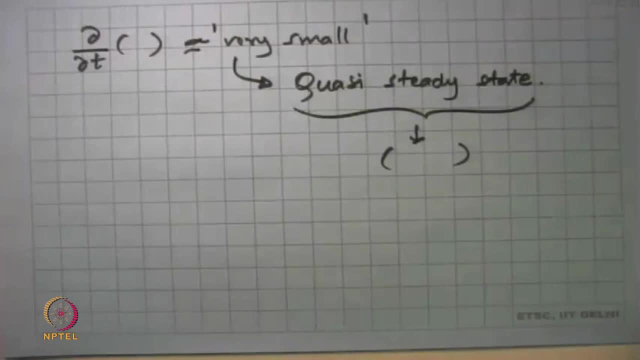 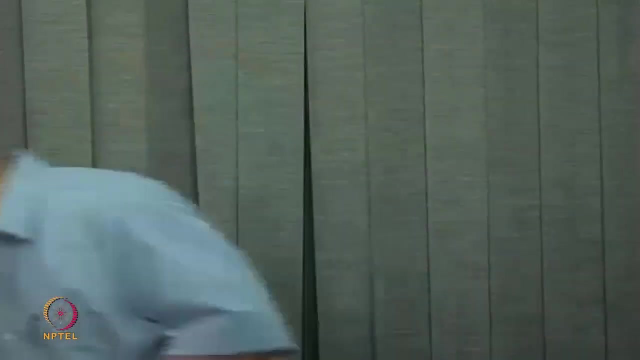 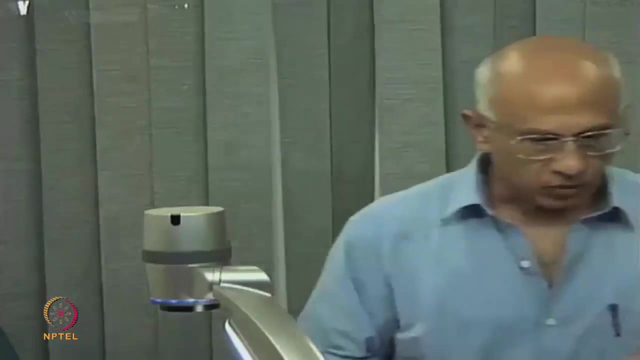 and what is the process that is? So this is an assumption that we make in many cases, in some case justified, some cases not justified. ok, So there are. there are couple of more questions. ok, So we have still got the reversible question is there. we will take that up. So 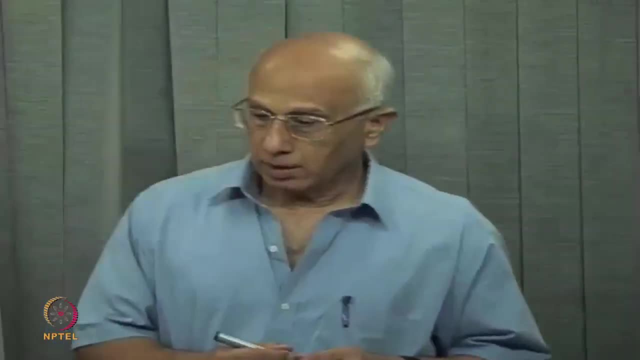 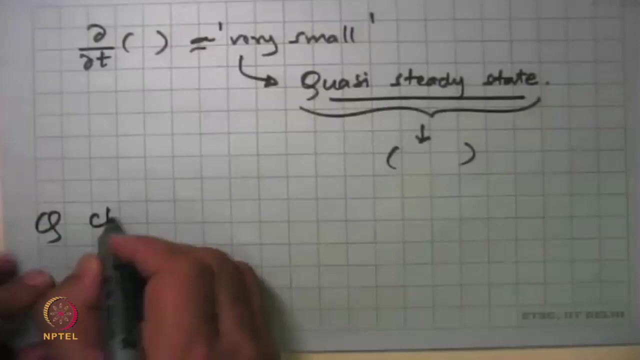 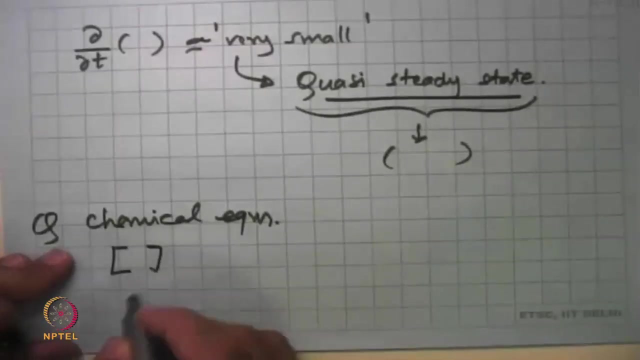 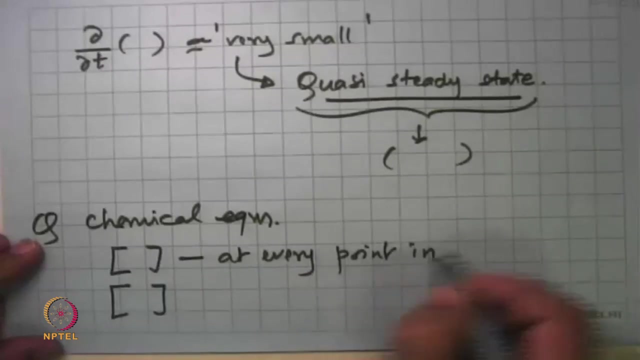 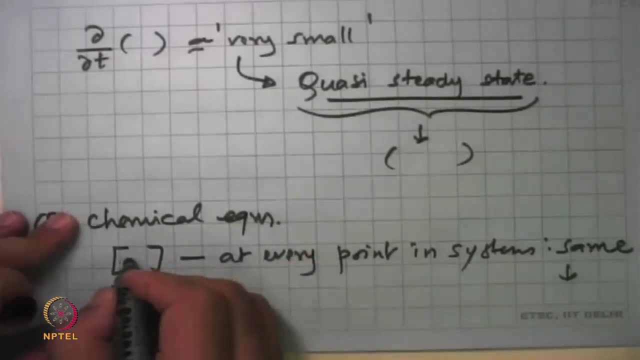 before that, please elaborate on chemical equilibrium. ok, What we are saying is That, what is chemical equilibrium? what we are saying is that if the concentration of different species at every place is the same, then the system is in chemical equilibrium. It means that we say that there is some chemical which was there. I will just call it chemical. 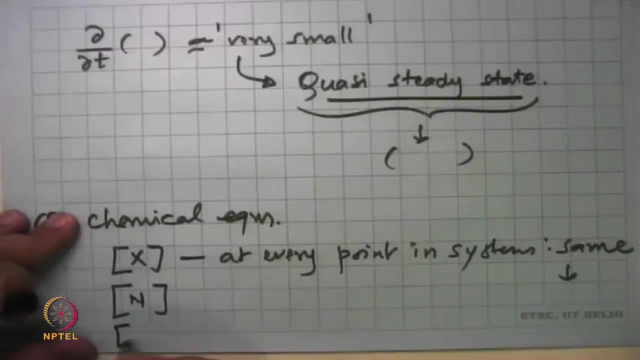 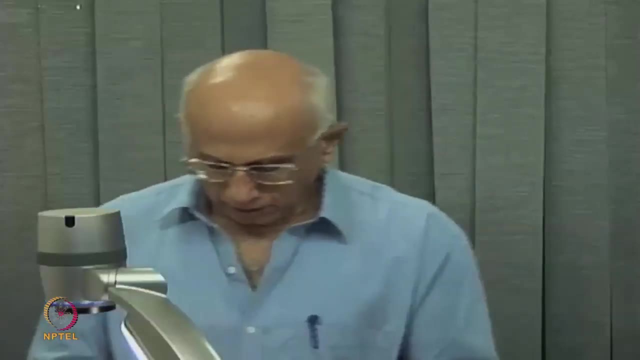 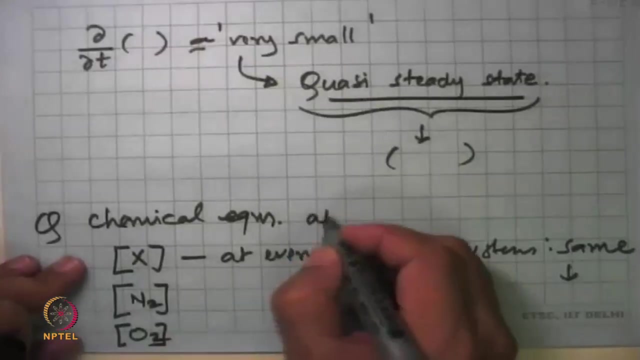 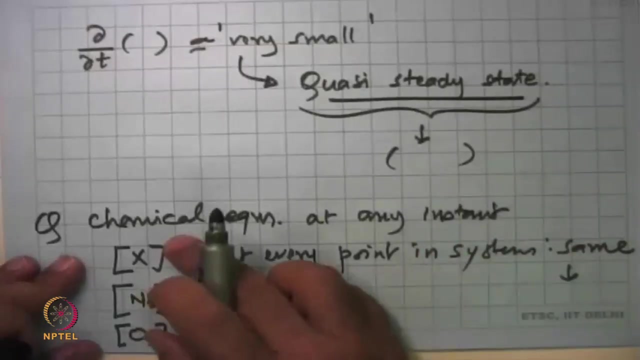 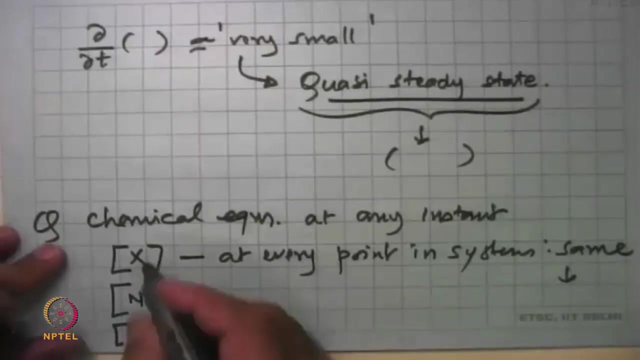 x, and in here we have n and we have o. If at every point in the room all these three concentrations are the same everywhere, at every point at any instant, Then the system is in chemical equilibrium. else it is not in chemical equilibrium. ok, So take for example that example, the mosquito repellent thing very close to the width of 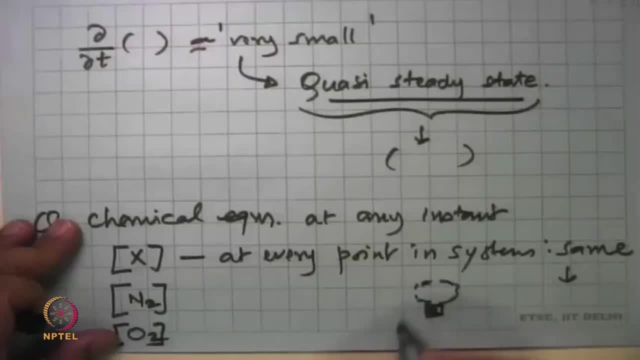 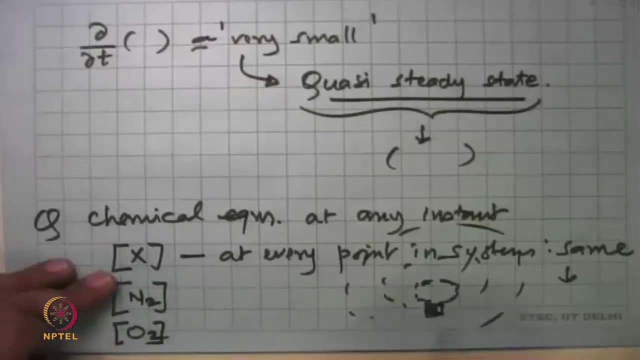 that thing. the concentration of that repellent is high. as you go out, the repellent concentration keeps on decreasing. This is what happens in the room. So here is the concentration of x, which is the repellent is more. here the concentration of x is less and far away. 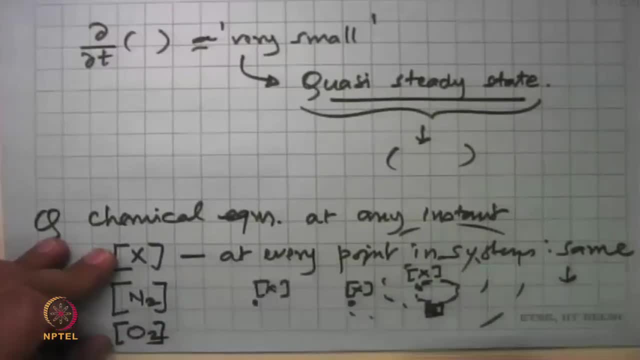 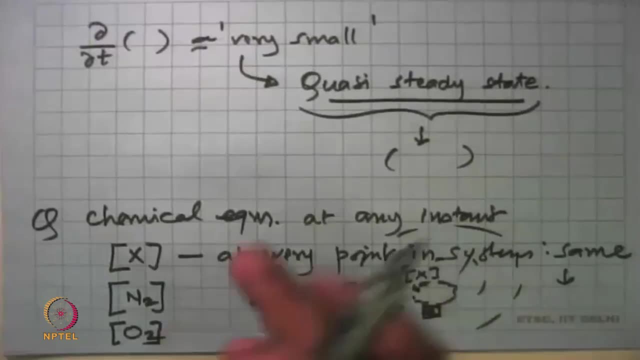 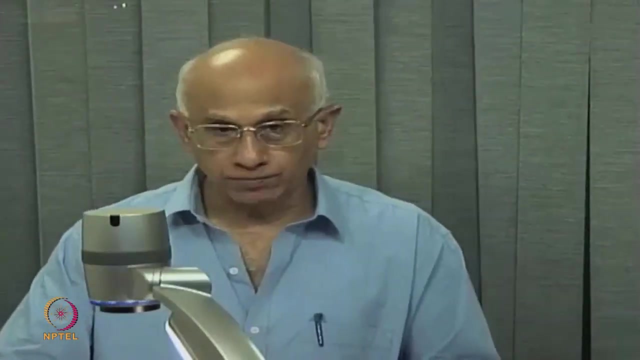 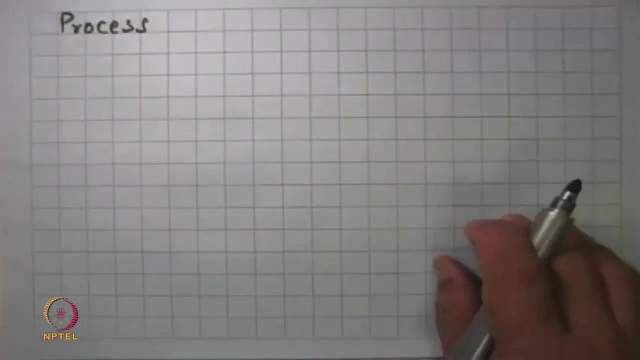 it is even less So in the same room. if this was different, then the system is not in chemical equilibrium. If it is same, then the system is in chemical equilibrium. ok, So we now come. go back to our process. Now we will look at the next most important definition, and this is the definition of a 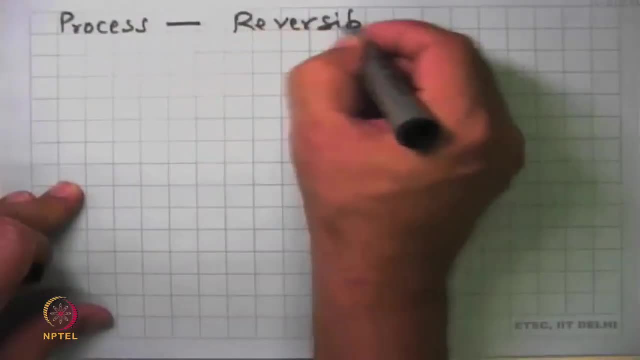 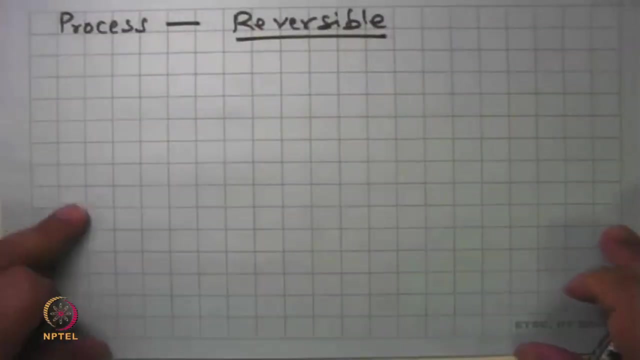 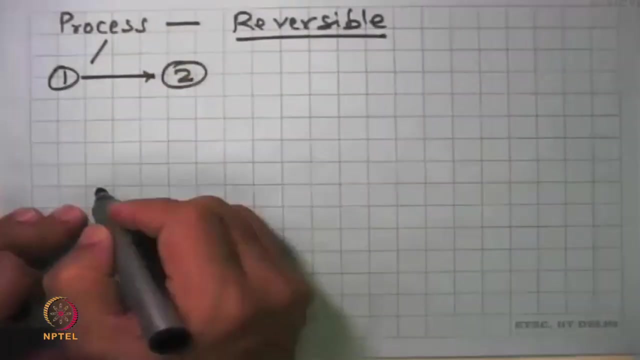 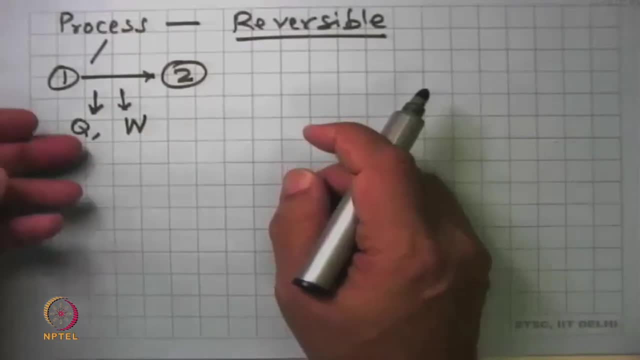 is also reaching at applying h In a browser function every 5 grams and in the browser function every 1 divided 0, a, x and y is equal to h And that is reflecting by 2.. overall OSE. we then figure out what happened there For the existing sogenanße state Glossary. 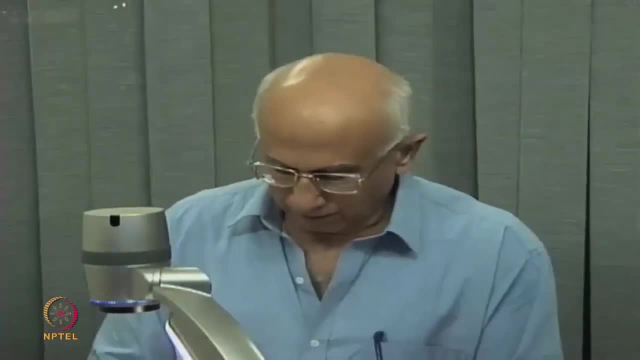 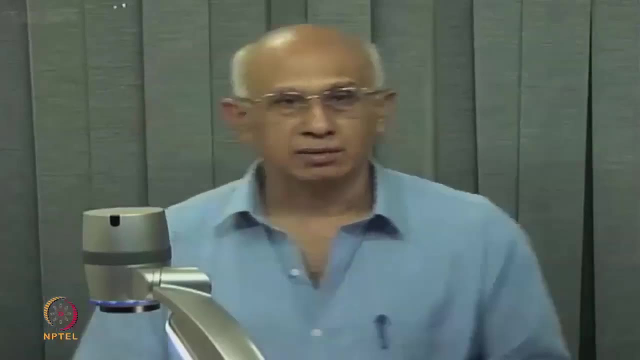 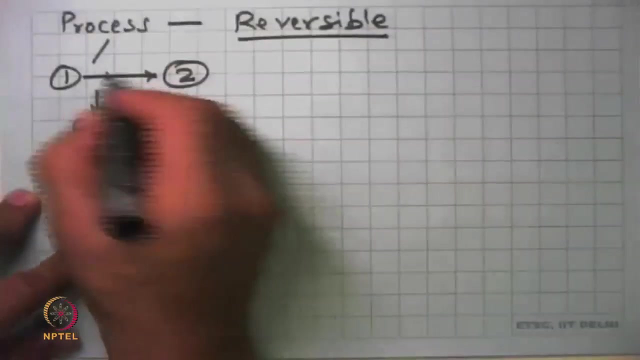 system, the opposite happens on the surroundings. So that means that in every process there is something happening to the system and something happening in the surroundings. ok, And we said that as process is reversible if at any instant we can reverse this process. 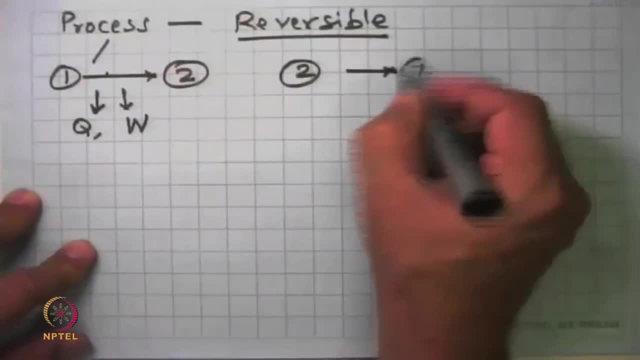 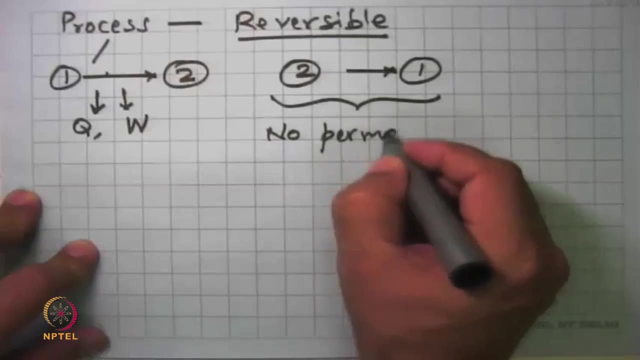 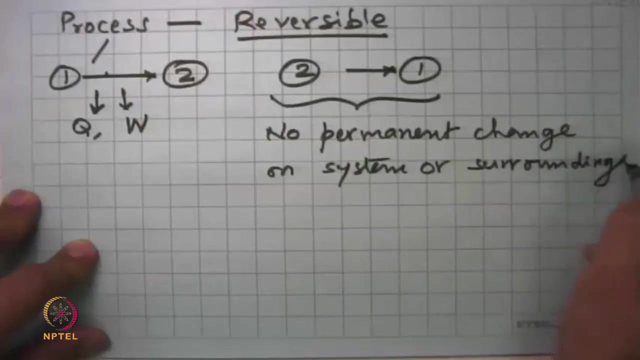 that means get back from state 2 to state 1, but in the process there is no permanent change on either the system or on the surroundings. ok, this is what we called the no permanent change on system or surroundings. That means both system becomes what it was before the 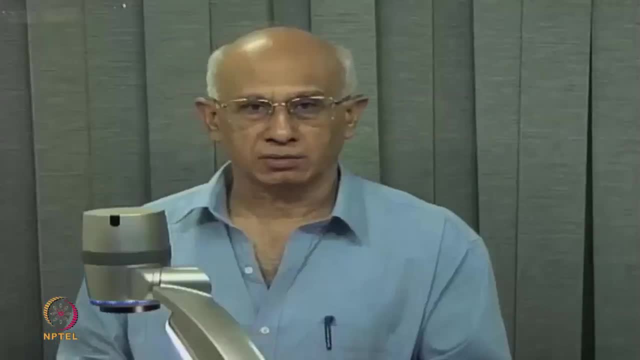 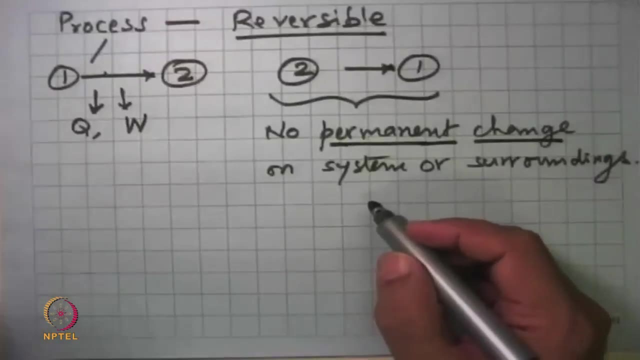 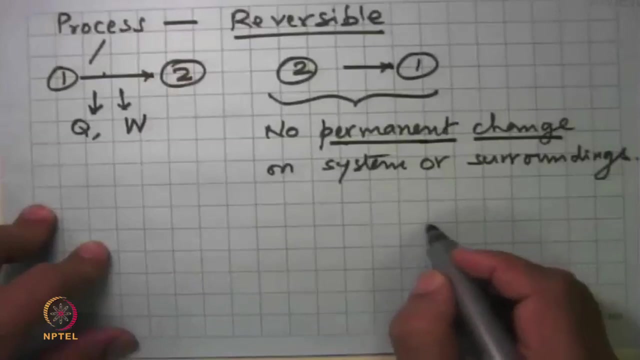 change and the surrounding also become the same before the change, Then that is permanent change. permanent change which not an instantaneous, one shot deal, but something that is always going to be there. So let us take a simple example. here is a, say, a block of material which is at temperature T 1, sitting in surroundings where T 2, where 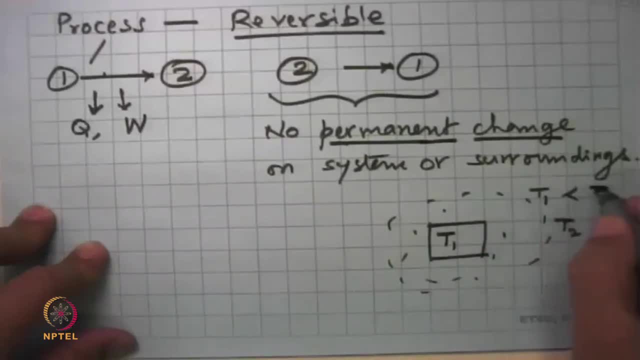 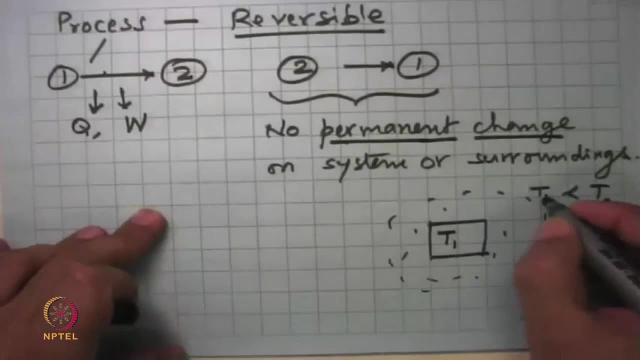 T 1. say T 1 is less than T 2.. So the body is cold. ok, or let us say the other one: T 1 is greater than T 2, is it all the same? So the first thing to do, to see here what. 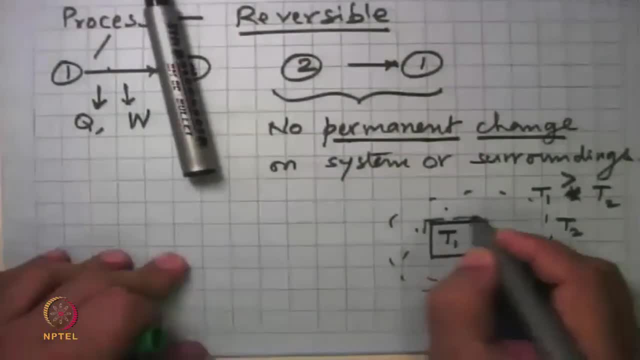 is the system and what is the process? the system, we say, is this thing and there will not be a face. So there is a body, there is a body, then there is a body. there is the body, there is a body, then there is a body. So there is a body and there is a body, and 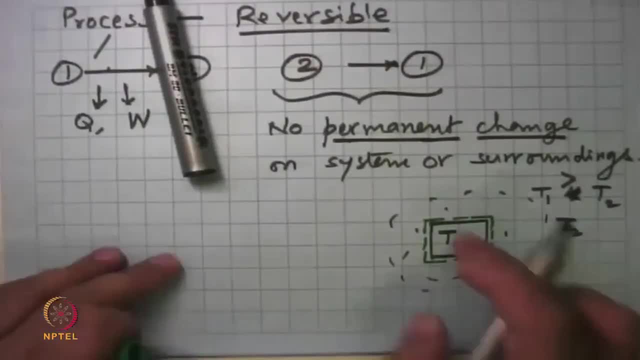 work transfer taking place. no mass transfer taking place in this. the only thing that happened was for the system, there was Q out and for the surroundings, which is now excluding this, everything else is surrounding. there is Q coming in, So this is minus Q, this is so. 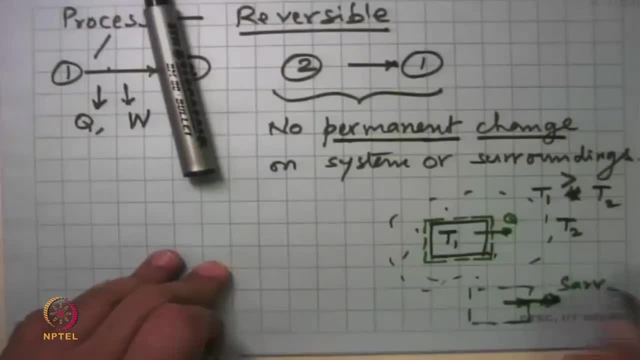 this is entering the system surroundings And say this was air. this air got hot and then we reached the state where, say, we started off with 70 degree C, T 1 and T 2 was say 20 degree C. after some time this became say 50 degree C and this became say 50 degree C. 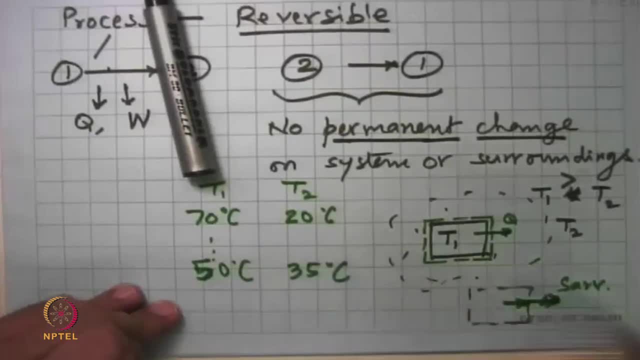 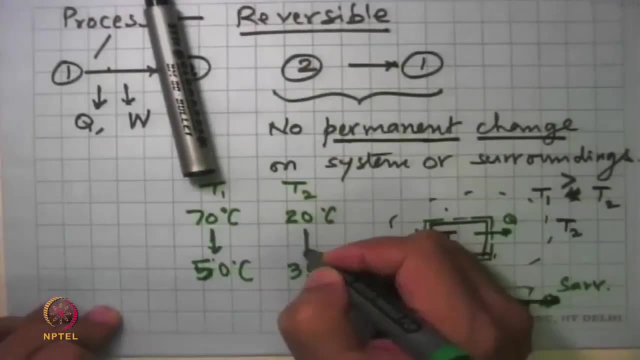 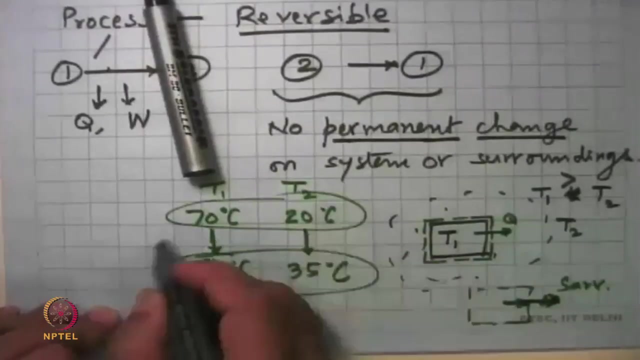 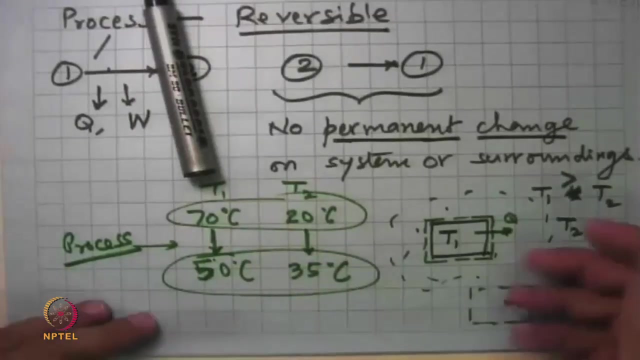 So the process was here, this was the initial state, this was the final state and this was our process. And now we say, is this reversal? and then say, well, how can I? I did not expect any work, we did not burn anything, nothing has happened. this thing, 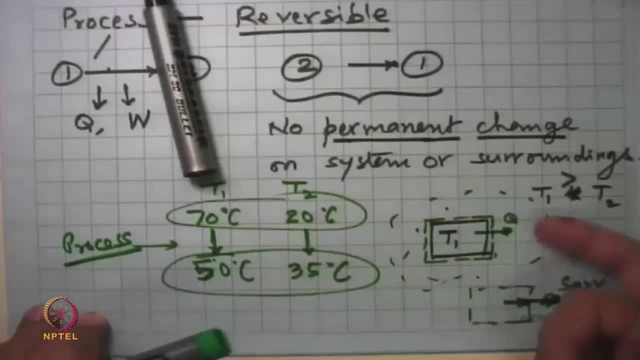 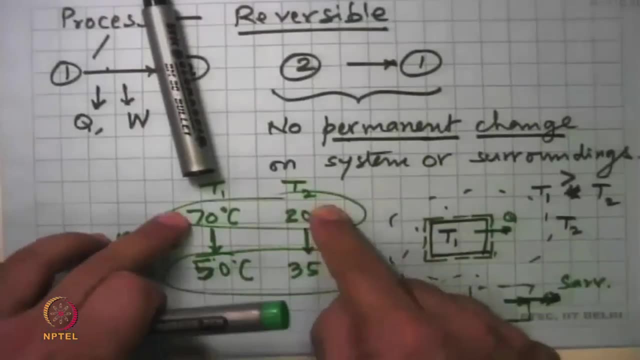 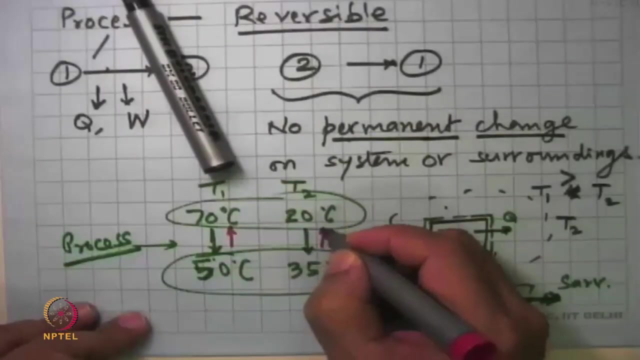 went by itself from here to there. Is it possible for this energy to go back this way, and we have heat there- So that this comes back to 20 and this goes back to 70.. So we are saying: can I by? can it by itself? this 50 becomes 70 and this 35 becomes 20.. And you all know. 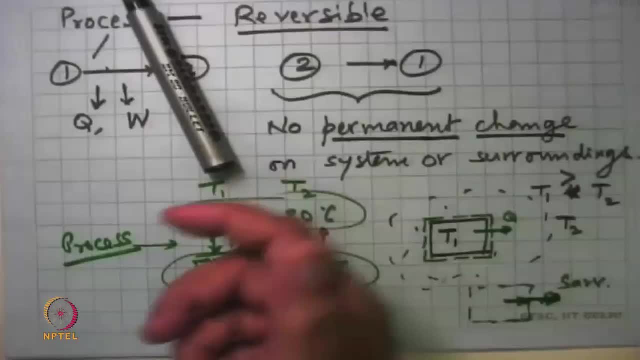 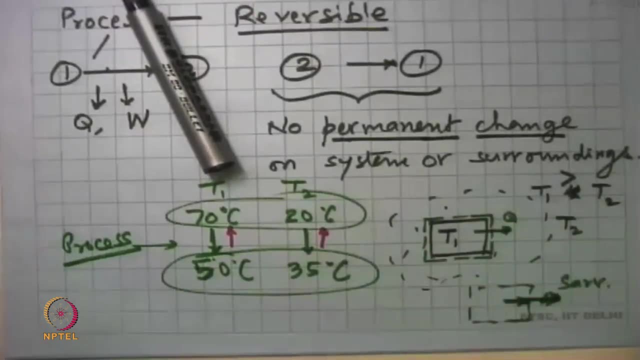 from experience that You cannot have heat transfer by itself, going from a low temperature to high temperature. You say: what is the next best thing I can do? Well, you said you know, if I want to bring system back to its original state, I need. 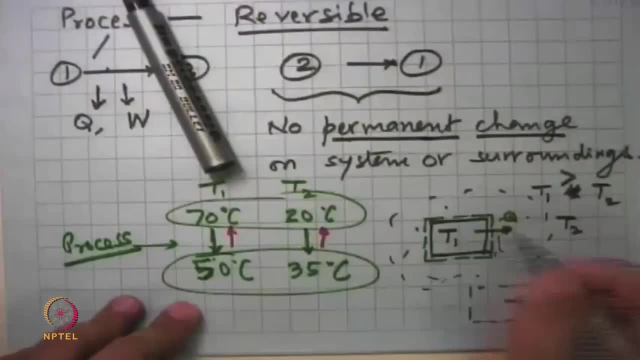 to have something in the surroundings which is higher temperature And say, ok, in around this I will burn some fuel. I have to produce gases which were. I want to get it back to 70 degree Celsius, So I produce a temperature of at least say about. 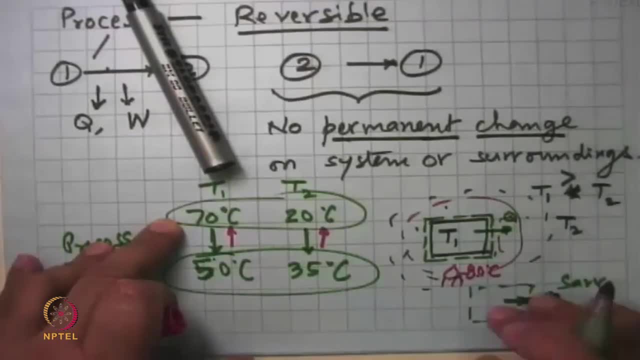 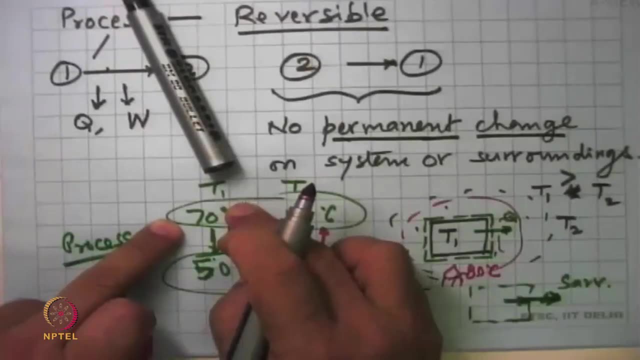 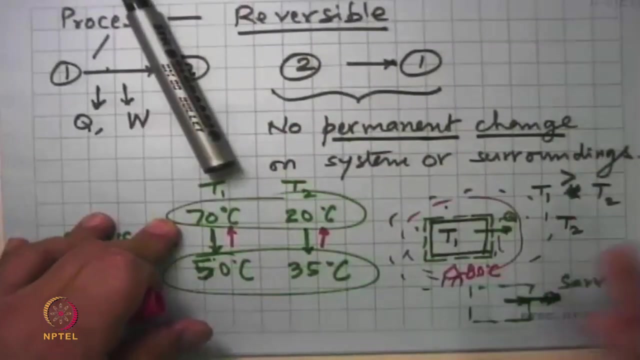 80 degree Celsius, or 90 or 100 degree Celsius. This will cause heat transfer back and T 1 will come back to 70.. So what is happened? The system got restored to its original state, It got reversal. but what happened on the surroundings? We got some permanent effect. 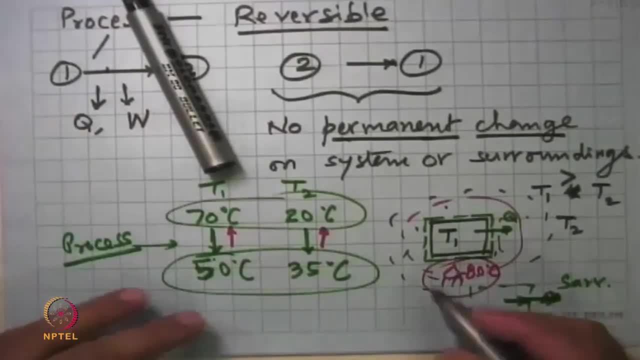 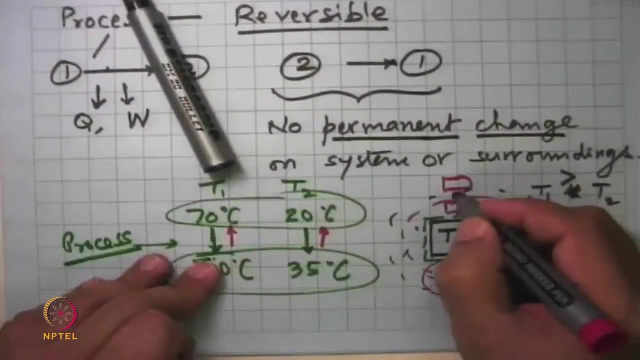 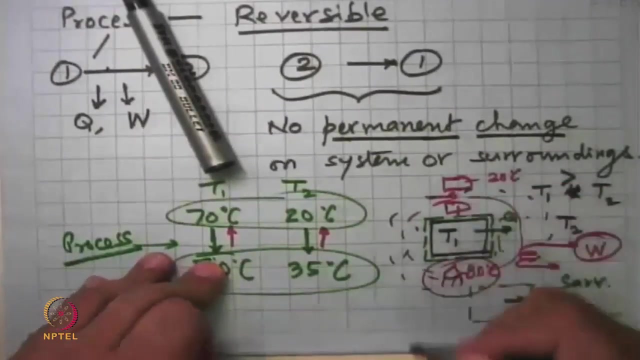 there in the form of, say, burning of a fuel or putting an electric heater which consumed electricity, or we put a heat pump, say like a refrigerator type of a thing, where this took electricity and took energy from a low temperature, which was 20 degree Celsius, and sent it out. All of these brought the system back to its 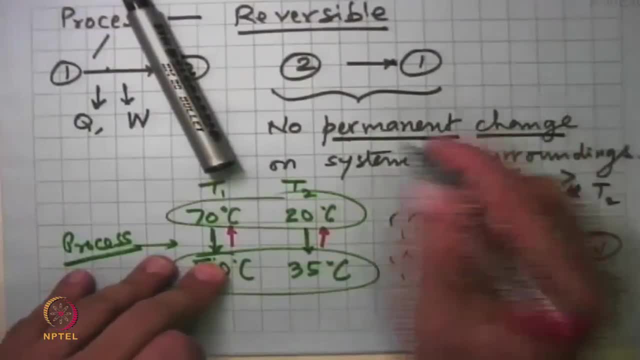 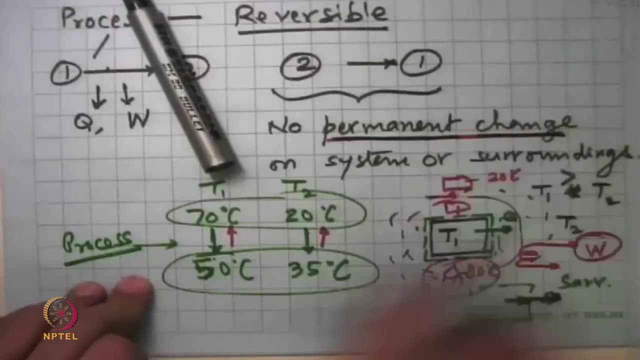 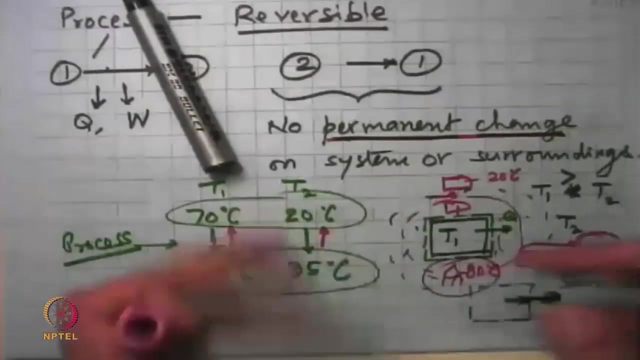 initial state, but the surroundings underwent what we call a permanent change. We expanded electricity to do drive the heat pump, or we expanded electricity to heat it up, or we burnt a fuel to heat it up that got depleted permanently in the surroundings, and so that classified. 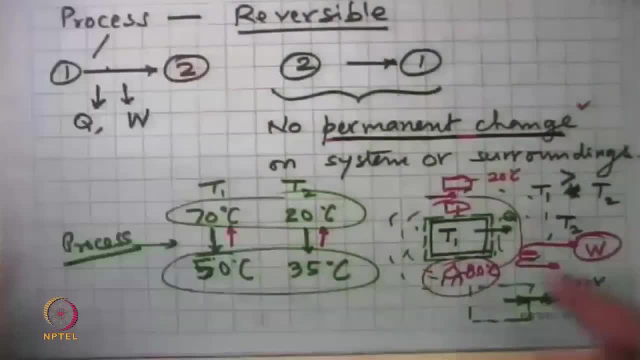 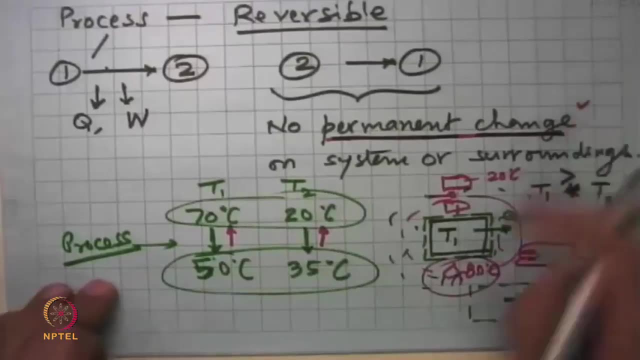 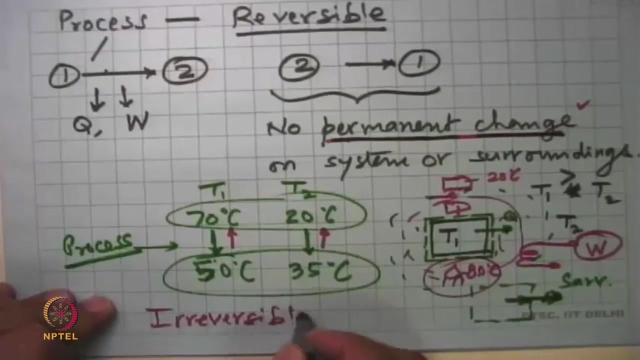 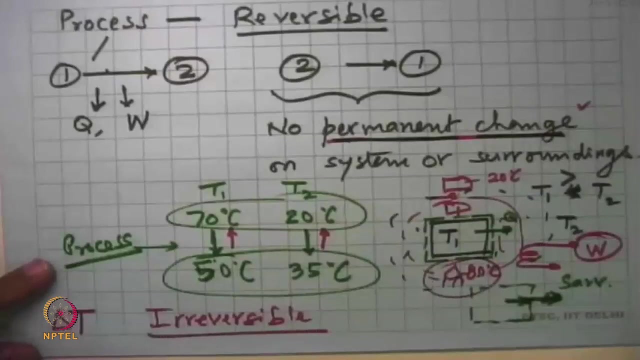 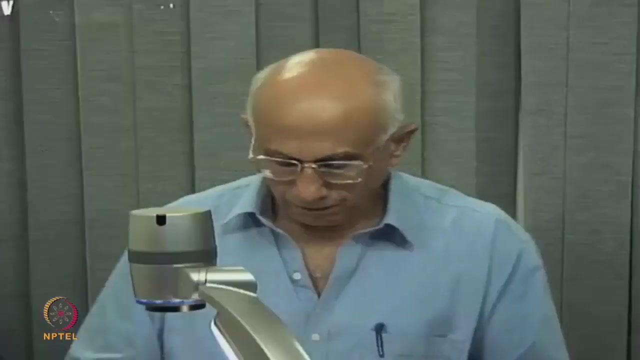 as a permanent change. And so if you could reverse the process with permanent change in the surroundings, and so this is not reversible or irreversible? That is one way that things happen, that heat transfer through a finite temperature difference is always irreversible. And you can argue yourself. 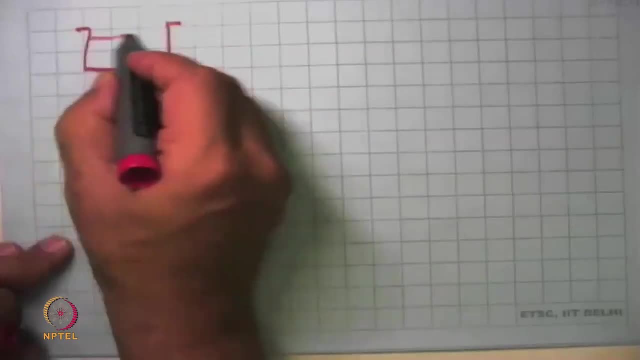 that I want to make a heat transfer. So I want to make a heat transfer through a finite temperature difference. Now I want to make a heat transfer through a finite temperature difference, And then I want to make a cup of tea. I have got so much water which I want. 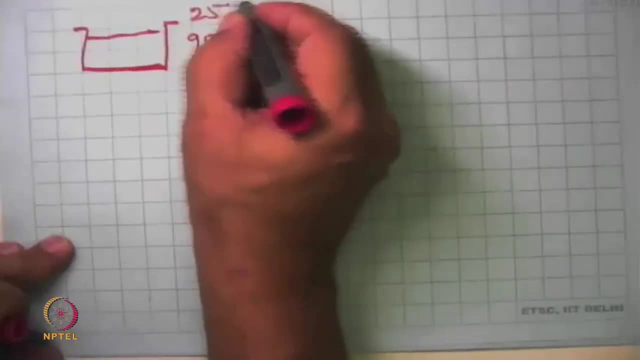 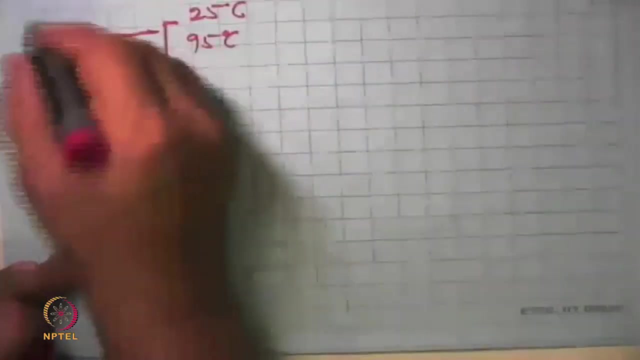 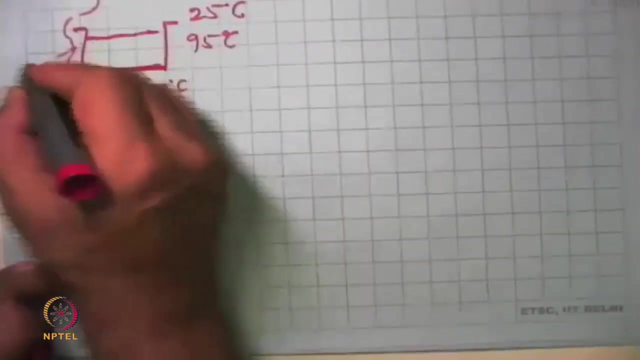 to heat to 95 degree Celsius. it is 25 degree Celsius. I have option number 1. I can heat it on my stove where the temperature of the gases that are going flowing around it like this and the flame itself is a 700 degree Celsius and the gases going here as a 200. 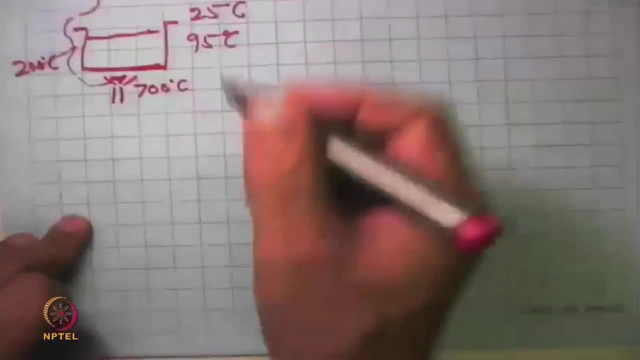 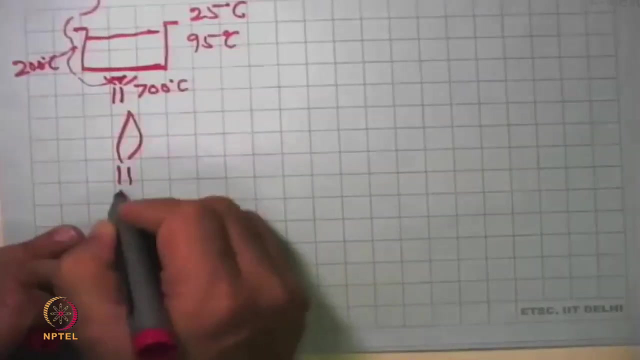 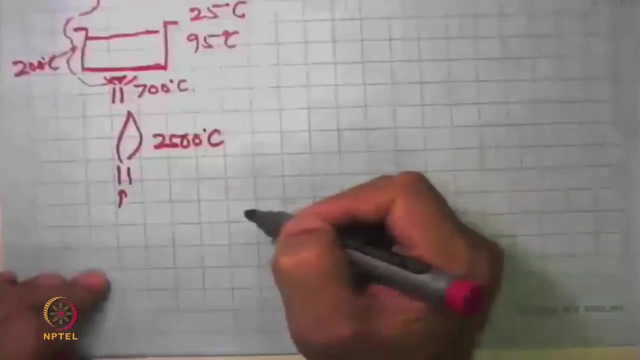 degrees Celsius. Somebody says: well, you know it takes some time. I want to do little more quickly. the fellow says: ok, why do not you put up an oxy acetylene flame over this? This is 2500 degree Celsius. just put it below, you will get heated up very quickly. Somebody: 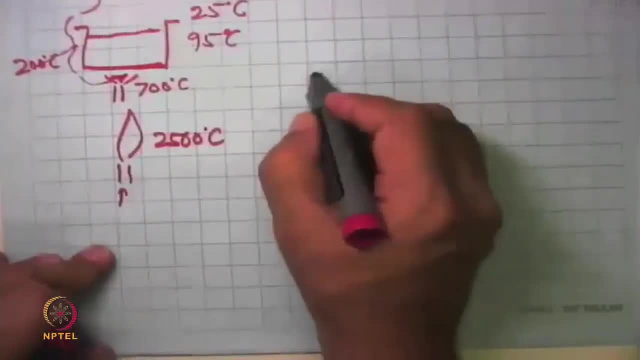 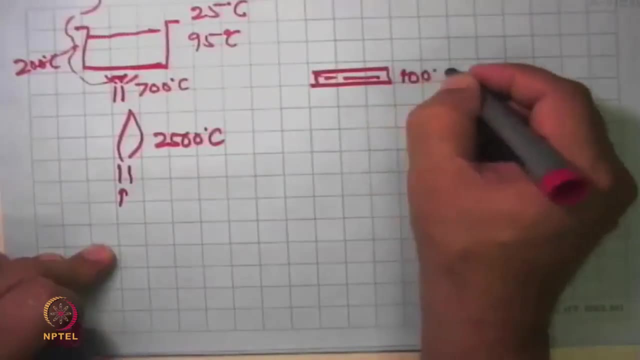 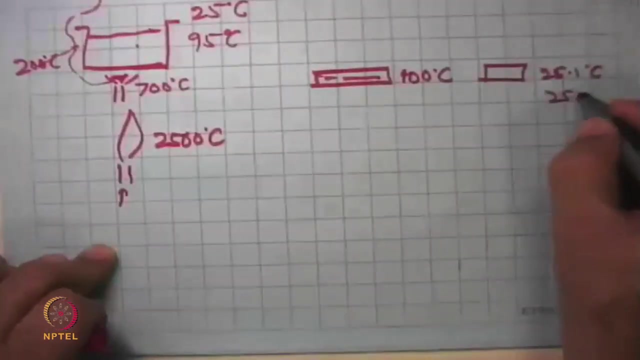 says: no, no, no, that is not good enough. I will just take a heater and maintain a temperature of, say, 100 degree Celsius on this. And third person says: look, when it is 25, I put a heater of 25.1 degree Celsius. When the water becomes 25.1, I will take this temperature to 25.2. 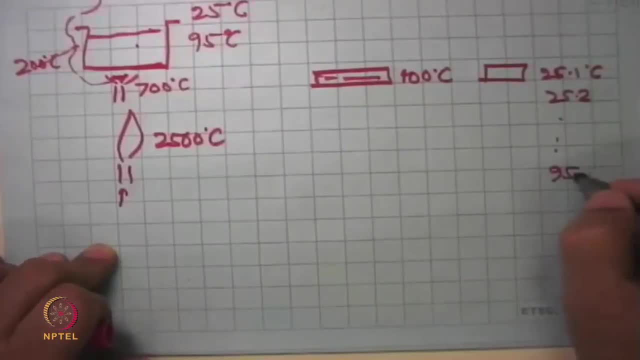 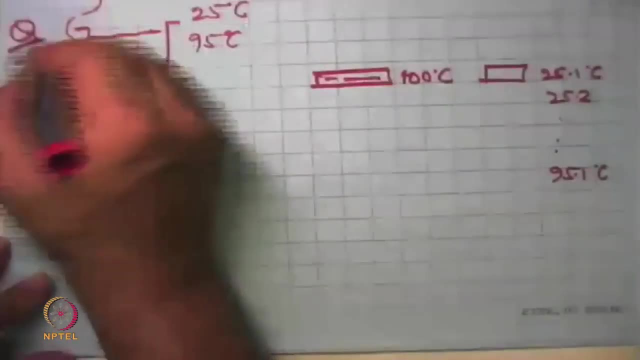 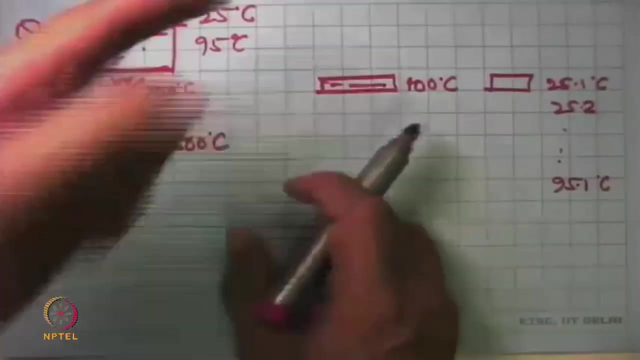 degree Celsius and like that. finally, I will get 95.1 degree Celsius and the water will become 90 degree Celsius. So I leave this question for you to think about. What is the thermodynamic implication of these things In terms of what we talked? 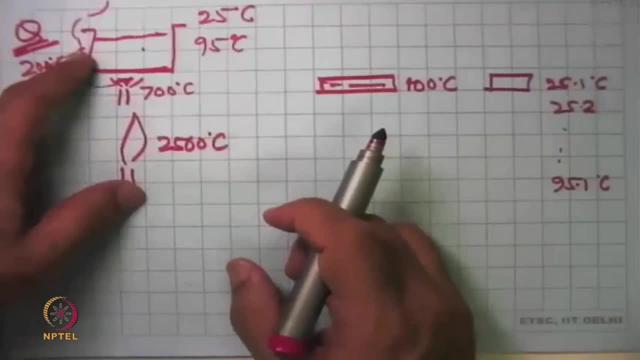 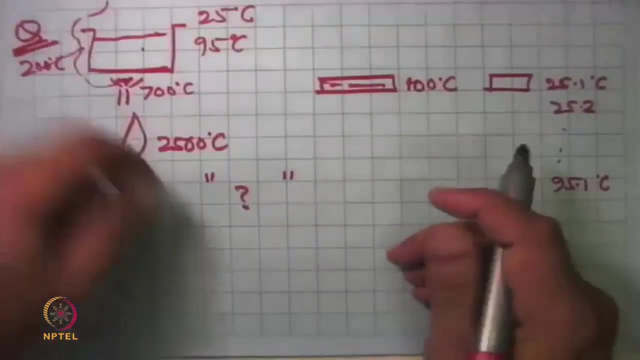 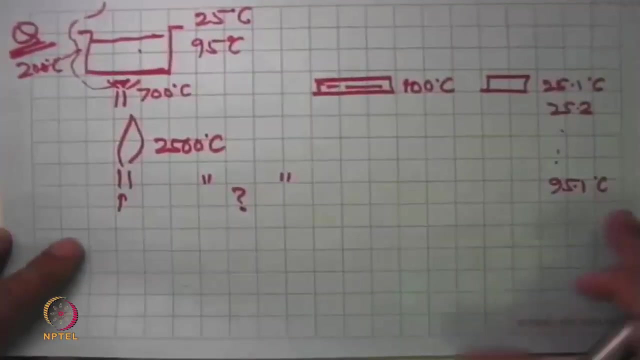 as irreversible heat transfer. we know that, were these, these are irreversible. What can we quantify as the gain or the loss because of irreversibility? ok, So this we will leave off and then argue then that if the temperature difference between the heat transfer happens, 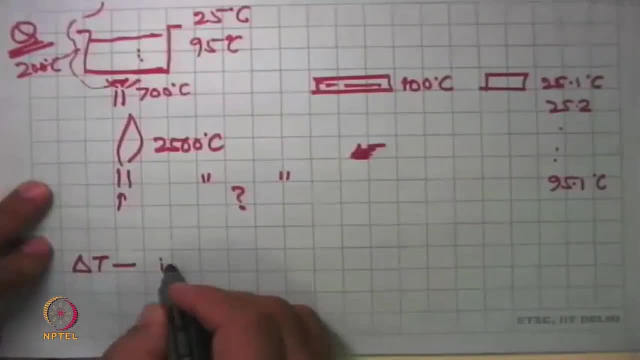 across a delta T which is infinitesimally small, and you are not saying what this means, then theoretically only we can argue this could become a reversible process. I am mentioning this because this is hugely counterintuitive. We know that heat transfer just cannot be. 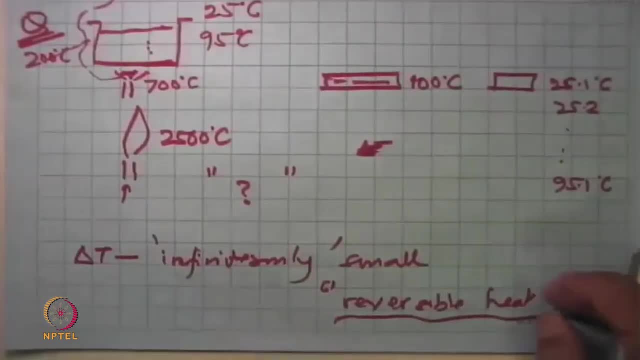 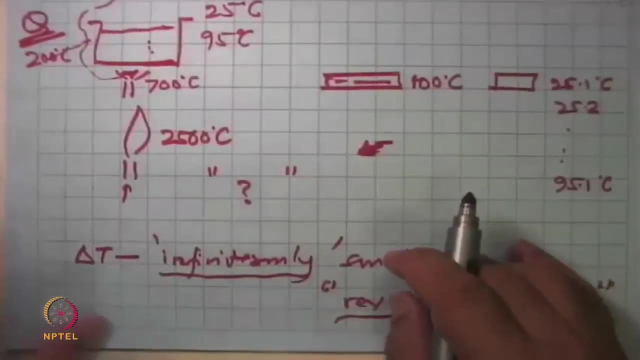 reversed without any permutations. So we know that heat transfer just cannot be reversed without any permutations. So we know that heat transfer just cannot be reversed without the change in the surroundings. but here is a concept, and it is purely a concept that we developed, that if by some means this temperature difference is exceptionally small, then with 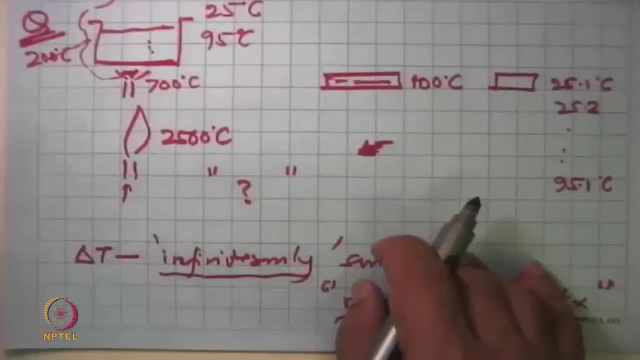 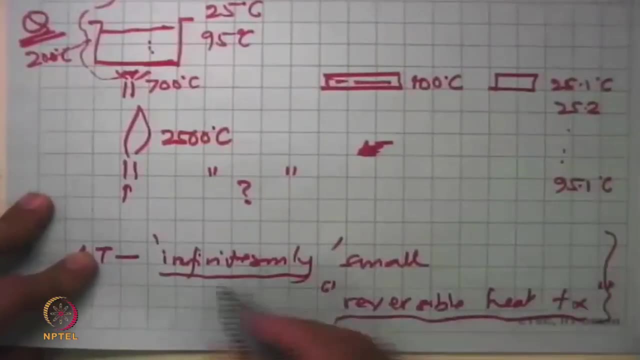 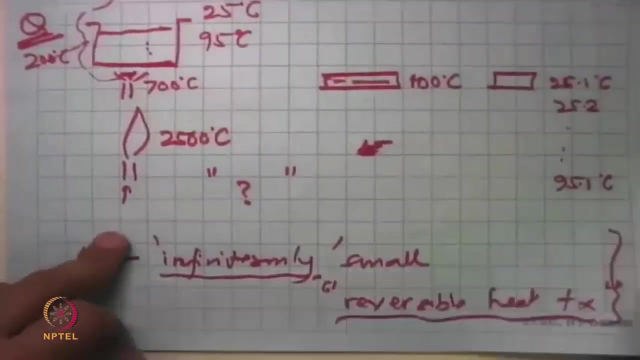 the exception: small amount of change in the surroundings. we can reverse that process. that is an approximation which is come out later on, whether very important approximation for us. There are pond. it is not very easy to appreciate this but the concept of reversible heat transfer in some way to some counter into it. but it is a useful concept. rarely. 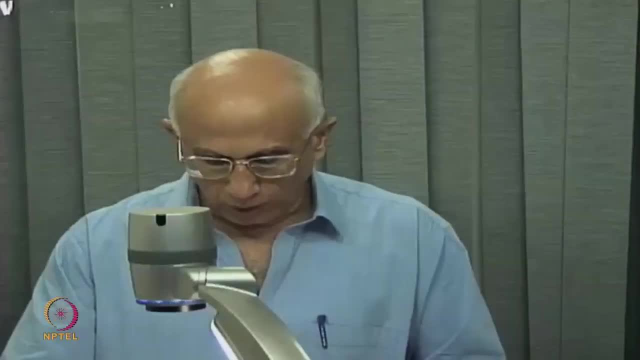 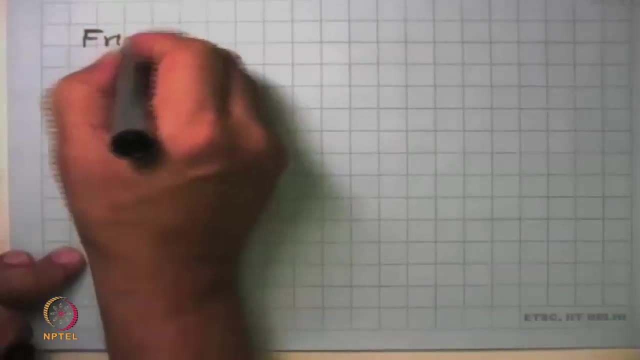 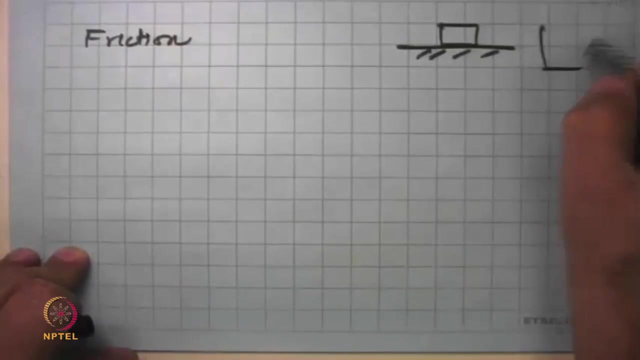 reality practically impossible to get. What are the other things that cause irreversibility? Friction, and this is not only friction of, say, a block set sliding on a table, but also we take, say, water, stir it and give it the water had energy because it is in motion, kinetic. 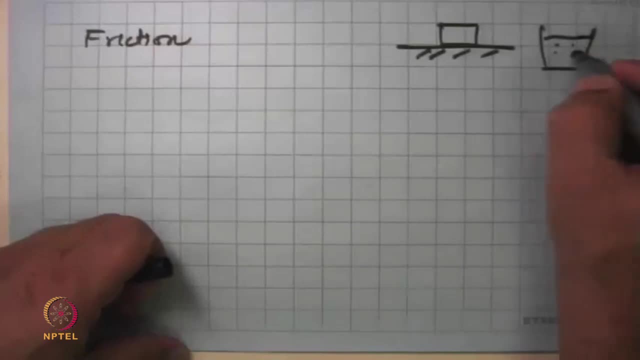 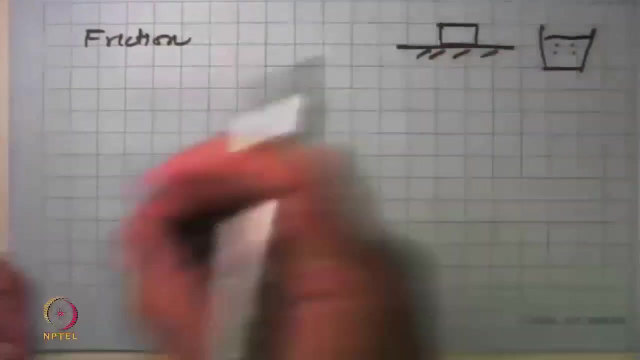 energy. Gradually it stops and everywhere it becomes 0.. So what happened Thing was that all of that got dissipated because there was friction between the element of the water itself. So friction is between solid, solid, solid liquid, liquid liquid. and when I put 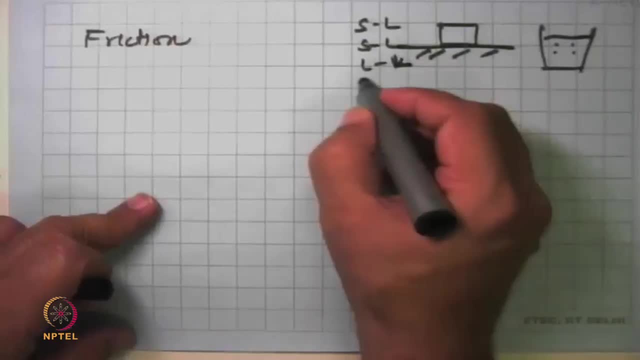 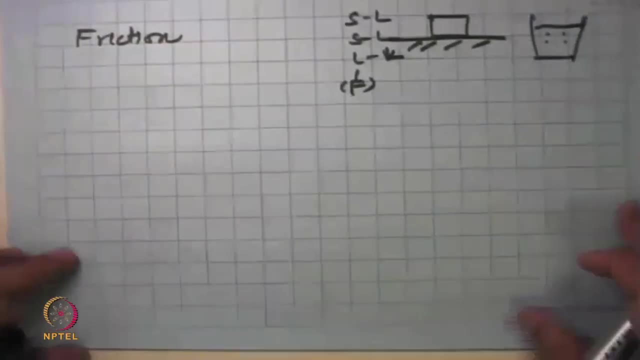 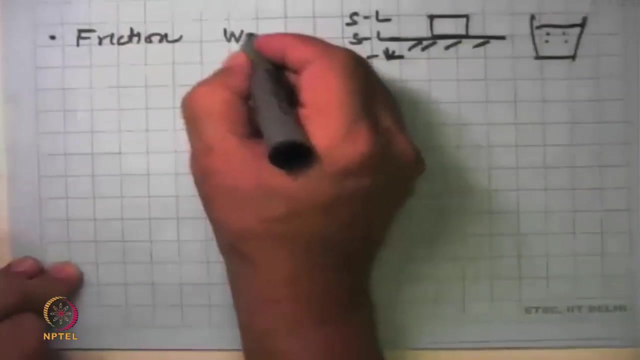 a liquid or liquid. the oil also can include a gas in it or a fluid. So there is friction everywhere, including the air. ok, So the friction causes, friction causes the friction. This because when friction happens, work is dissipated and it converted into heat. 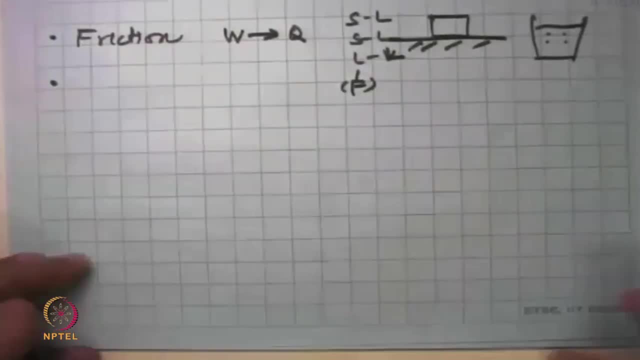 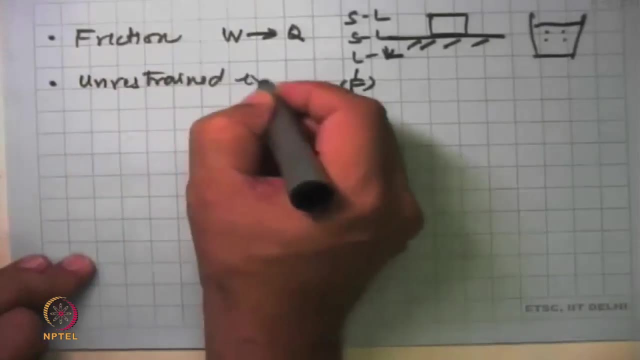 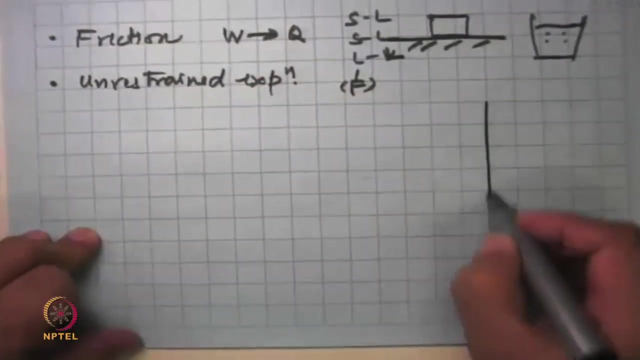 and just cannot get the opposite thing down. Then there is unrestrained expansion. So we say unrestrained expansion is irreversible. So let us talk about what becomes restrained expansion. So that is a piston sitting there. So that is a piston sitting there. So this is a piston sitting there. So this is a piston sitting. 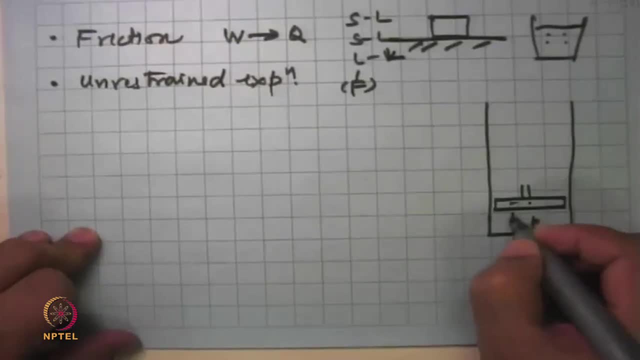 and we are. there is a pressures here. this is producing a certain force and this is a force. this is just about matching this force. So this thing is pushing against this force and the piston moves a small distance and comes over there. The pressure inside goes. 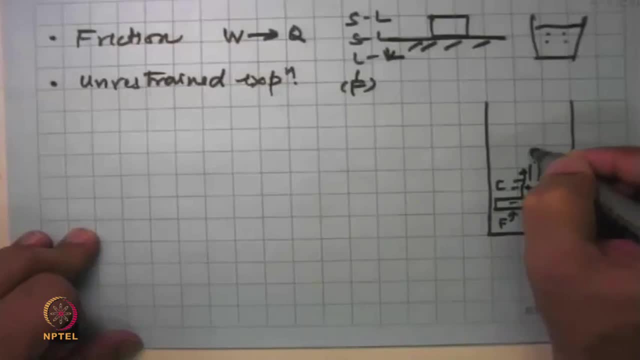 down, and then it pushes that force and goes back. So there is a very, very small steps in which the force that is acting on the piston is practically the same as the force that the fluid is exerting on it. So this force, which is the restraining force, 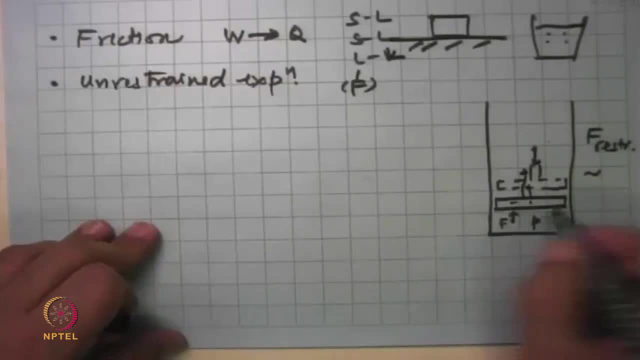 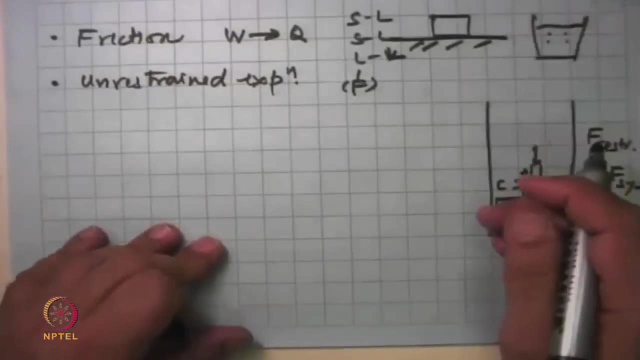 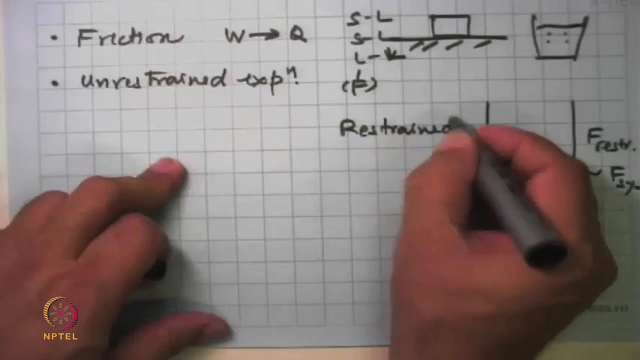 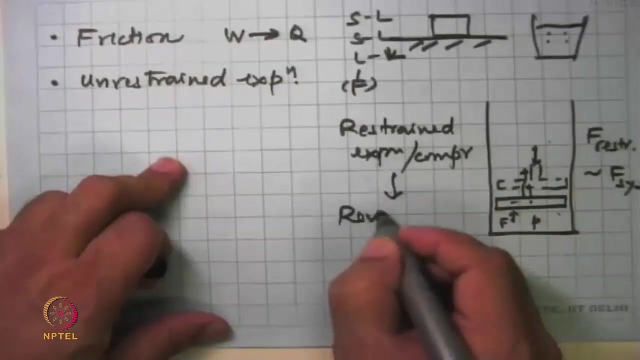 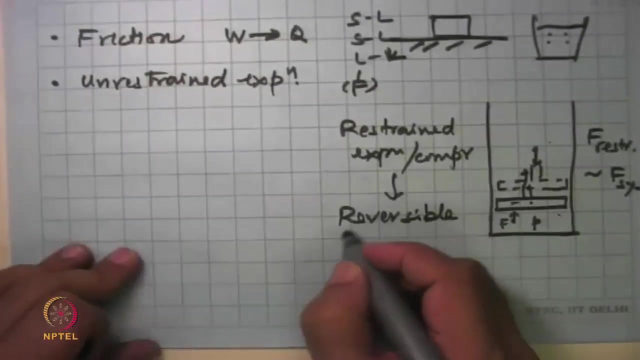 is very much equal to the force that is exerted by the system on the piston, and if the two are pretty much the same, whether it is expansion or compression, then this becomes an example of restrained expansion or compression, And this we say is reversible. ok, So this is reversible work. what is unrestrained expansion? 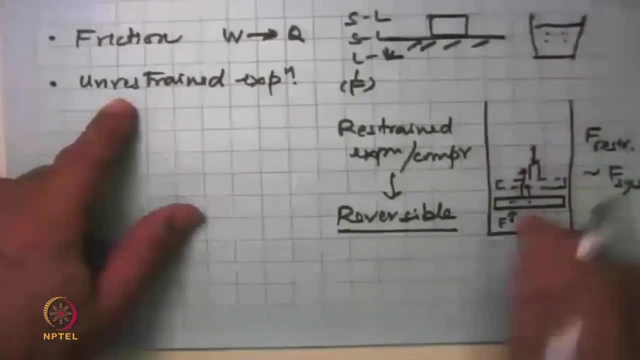 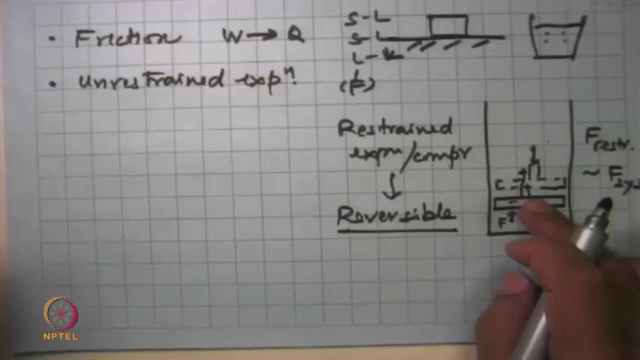 when you, you are holding it down with certain force at this point of time, and then suddenly we just let it go. So we know that you do not let it go. So we know that you do not let it go. So we know that you do not let it go. So by the bicycle pump compression. 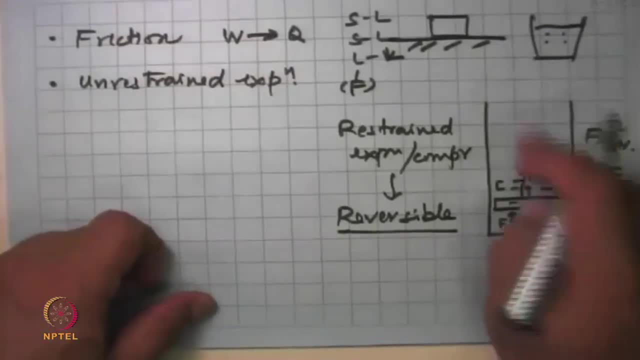 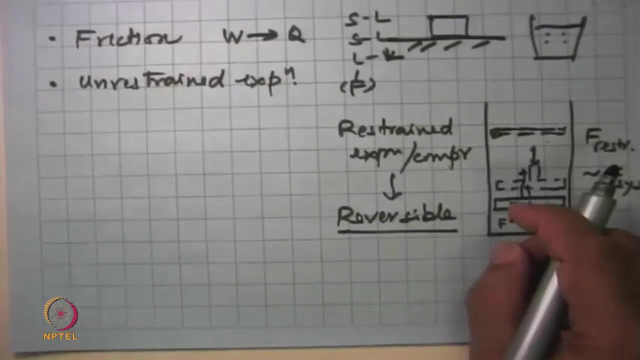 let it go. it just go up and down, pops a few times, So it will go up and down and finally it will settle down somewhere there which would have been in its equilibrium position anyway. but during this process, the only work it did was to move the piston. if the piston 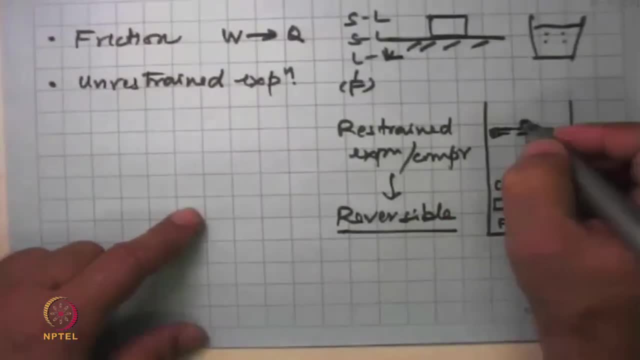 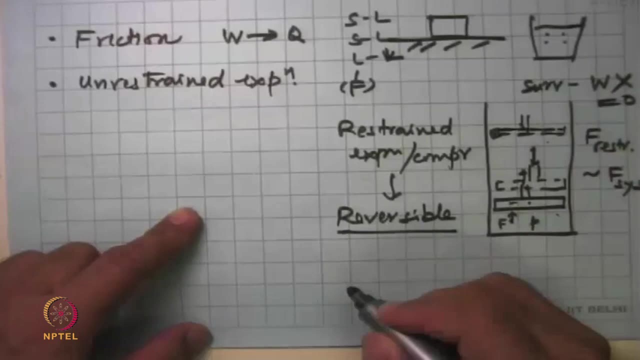 at no mass. it did do anywhere. The surroundings: there was no work on the surroundings. work was 0.. But you can want to get it back from here, The have to there. we would have to do work on it to get it back to the initial state There. 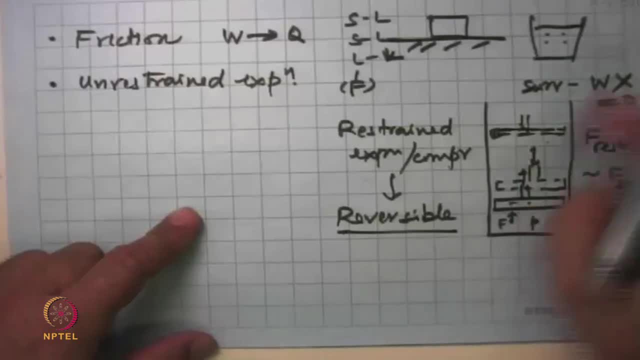 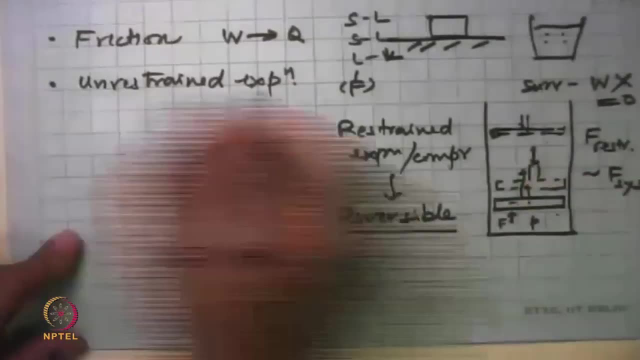 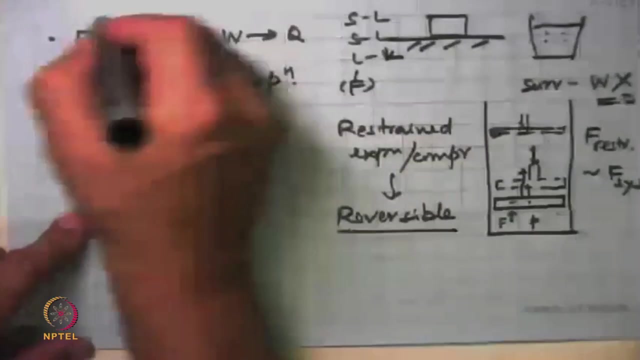 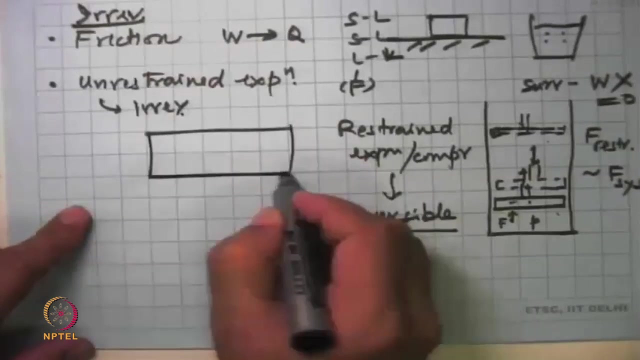 we would have to expand work, and so, while unrestrained expansion, we got no work to restore the system back to its initial state. we have to do work, and that is what makes unrestrained expansion irreversible. This was friction wall, also called irreversible. Another example of unrestrained expansion is that we take a chamber in which this side 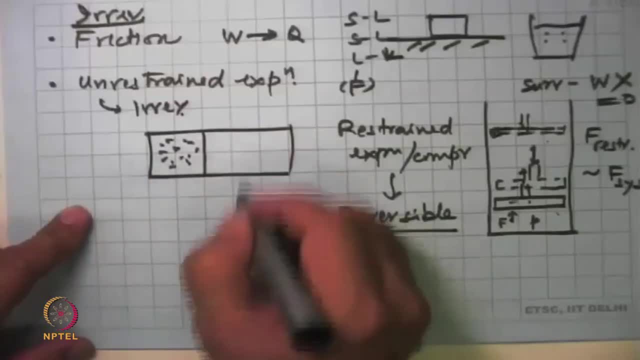 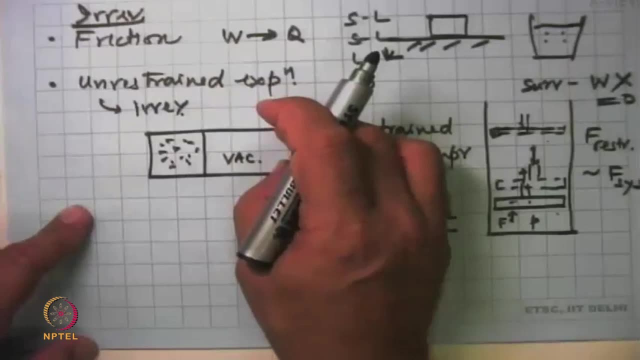 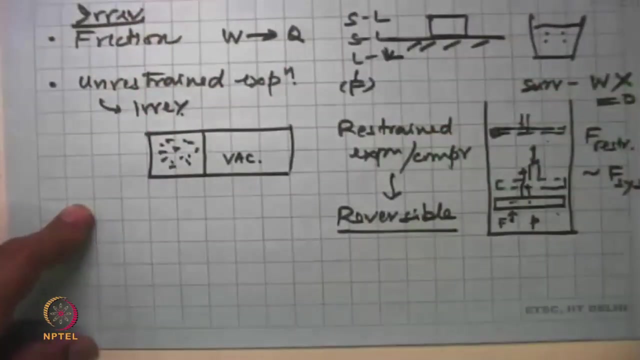 there is a gas and this side there is vacuum And we ru rupture these. this gas expands. it does not do any work. but to put it back, we need to do work to get back to the same thing, and that work is permanent change on the surroundings. Then there is mixing. we have to do the work. 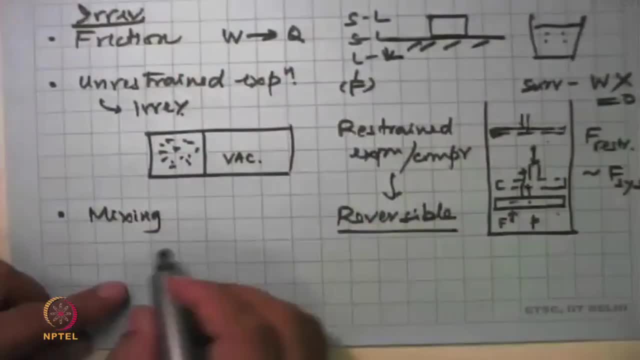 on it. Mixing means mixing of two different species. If we say that I am going to put, say, any gas into the air, the two will mix and say now I want to remove the separate the two out, but naturally they will not come. we would. 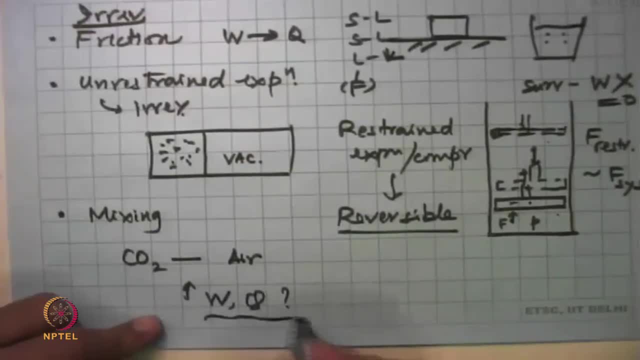 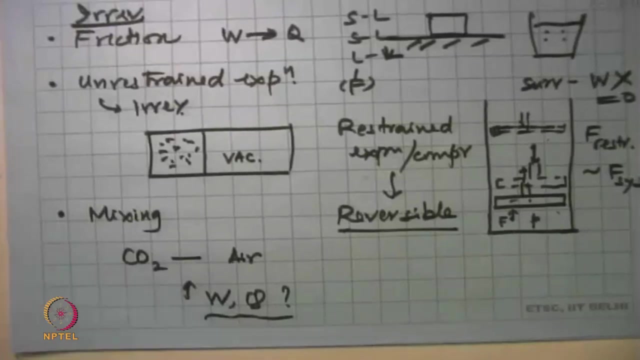 need to put in some work, maybe some heat, and these will be permanent effect on the surrounding, and then only you can restore the system back to its original state. ok, So these are the two. Some of the things are called irreversibility. ok, there are questions, so we have few minutes. 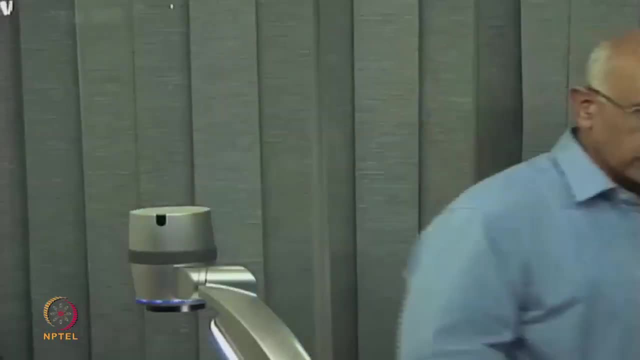 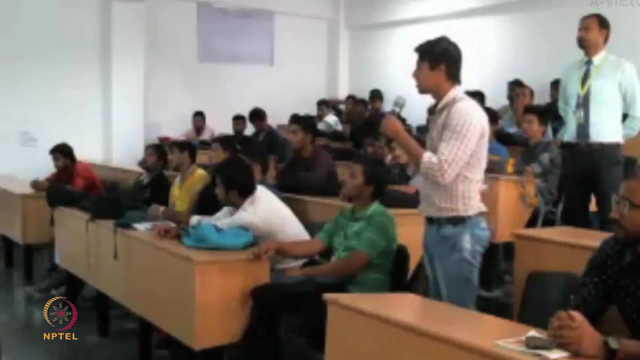 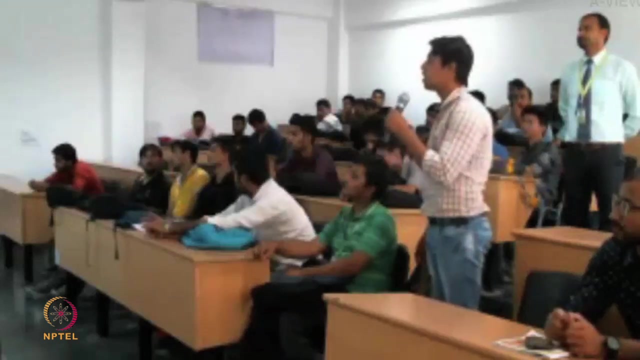 left. I take some questions and the rest I will then respond to it on the way. Good morning, sir. My name is Manjit Singh. I am a fourth year mechanical student at Dronacharya College of Engineering and my question is, sir: can we use biogas as a fuel in internal combustion engine made from cow dung, and what? 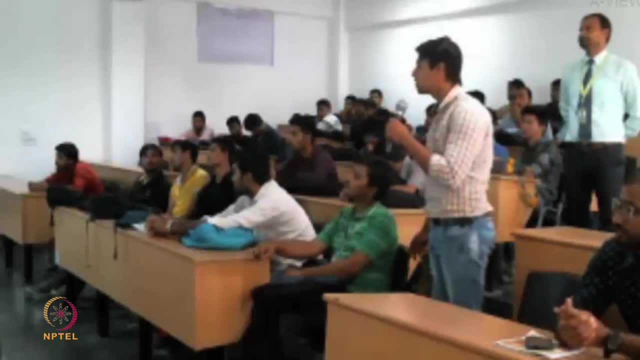 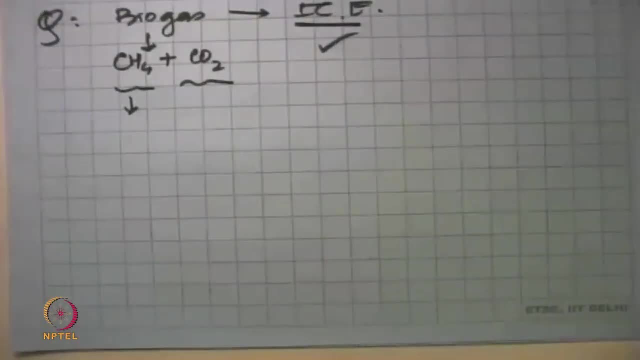 done and it is fairly standard technology. it is already available commercially, So there is nothing new to be done on that. gas engines are available from most manufacturers As far as the mileage and emissions go, there you can read up on the literature on the web. 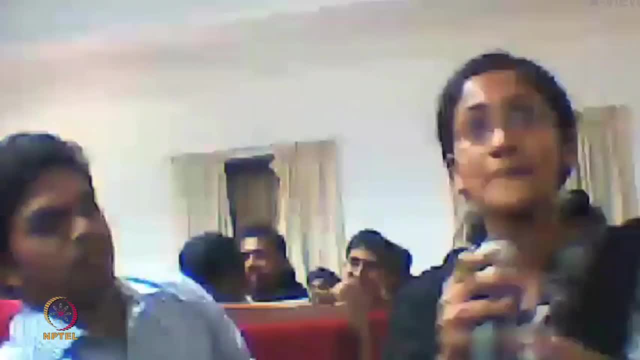 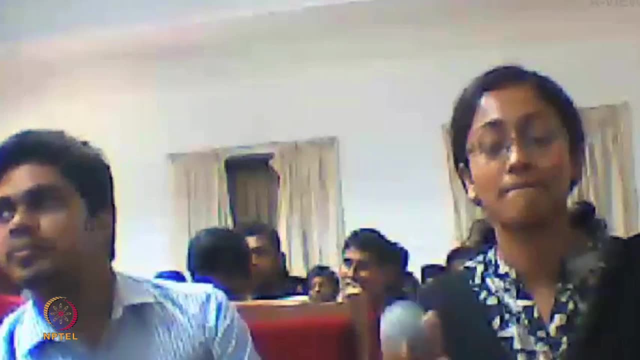 I will not go into it. Ok, I will not go into it. Data is there. Yeah, We have already studied that heat and work depend on the path. why is it so? Say that again. Yes, Heater, Say that again. 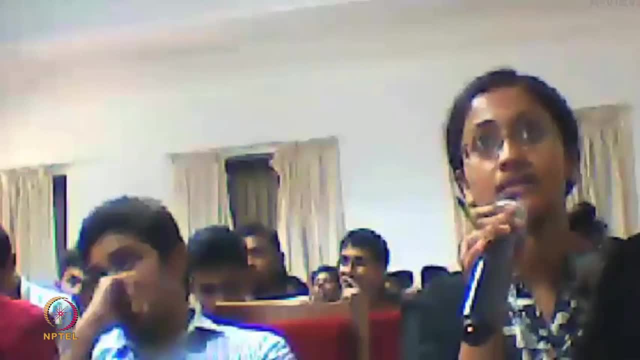 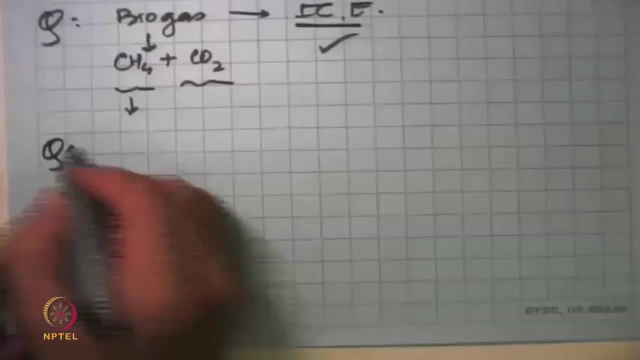 Heater, Heater. Heat and work depend on the path. their path functions, Ok. Ok. So the question is: I am: I mentioned that heat and work will be associated with a change of state, So we have gone from state 1 to state 2 and I also mentioned that when this change of 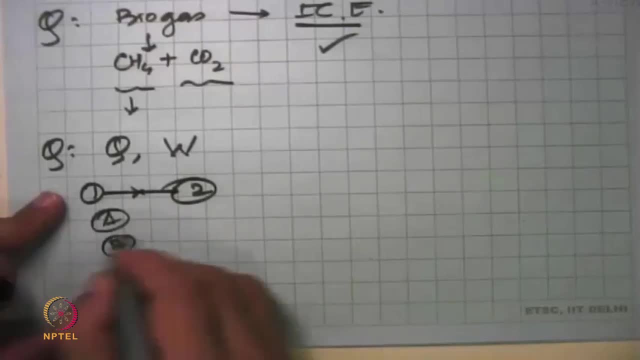 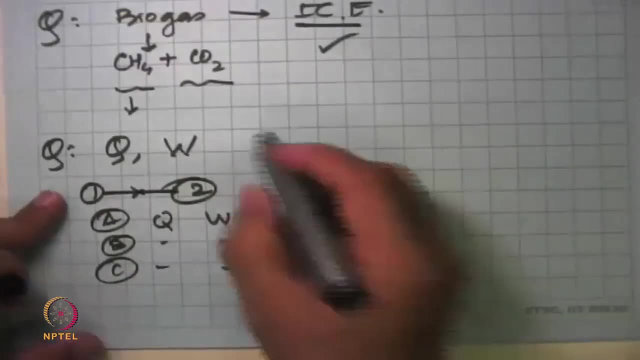 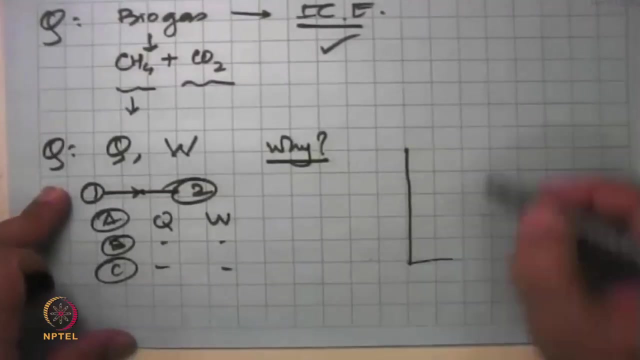 state takes place. depending on the path that one follows, it will decide that Q and W in each case is going to be different. The question is: why is this so? Ok, So I will give an example and then you will see that. suppose I have a gas which has to. 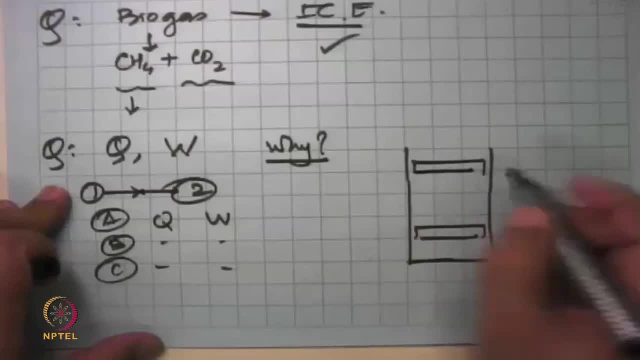 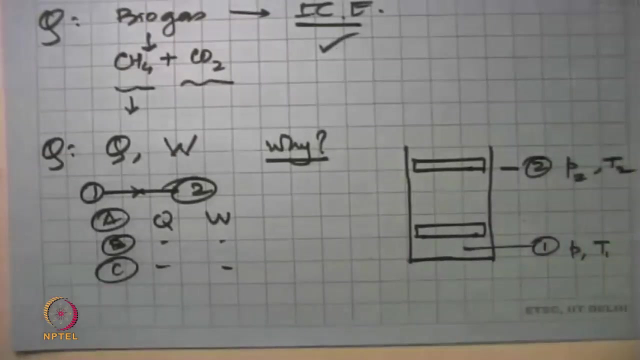 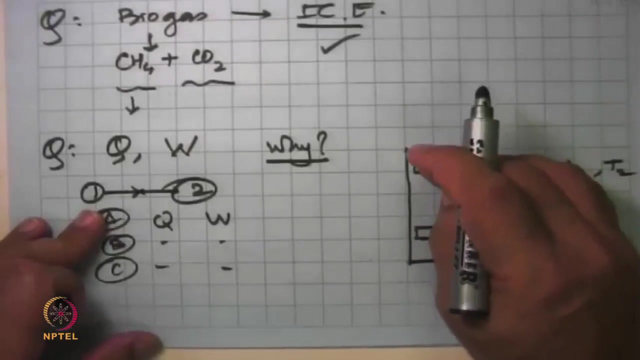 expand from here, and this much is the volume change and my in the initial state 1, there is certain pressure and say certain temperature, T 1, and then it reaches this state and here you have T 2 and T 2.. To get from here to here, one could do is expand this and then, if the temperature does not match, 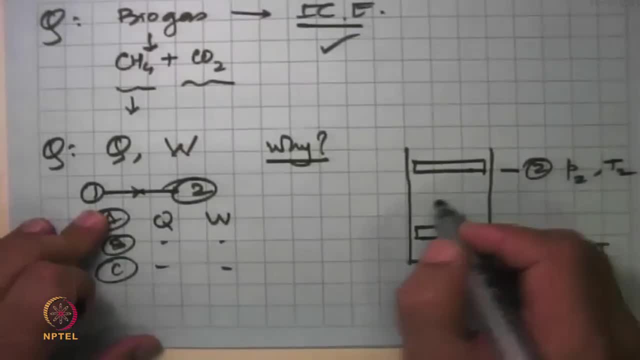 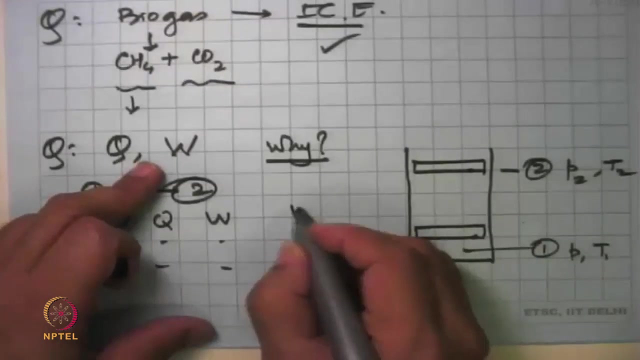 with the T 2 that you have, you can either add heat or you can cool it, or alternately, you can first heat it and then allow it to expand so that it becomes cool. So you can. at least two things are possible: That you first do some work and then gives plus some heat, or first heat it and do some. 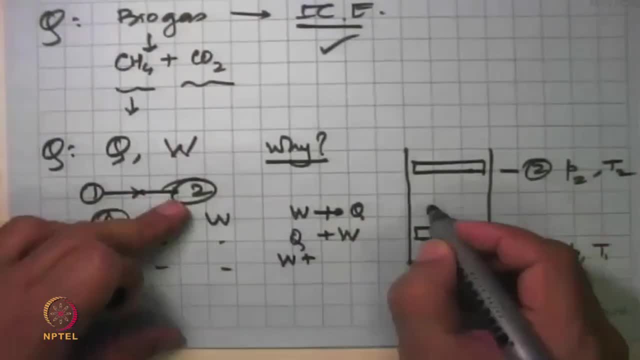 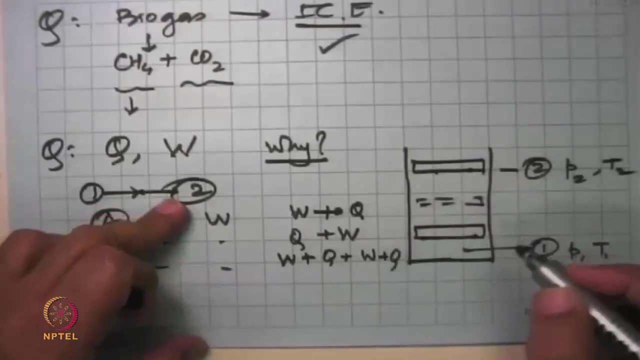 work, or any combinations of these: some work that brings it up to here, then you heat it, then some work, then some more heat, and it brings it up to here. So what is happening in each one of these cases is that the final state is the same. 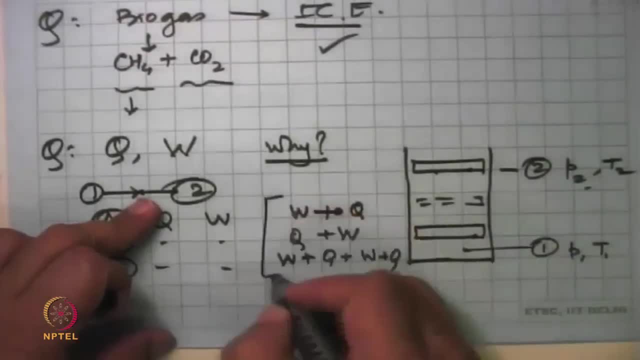 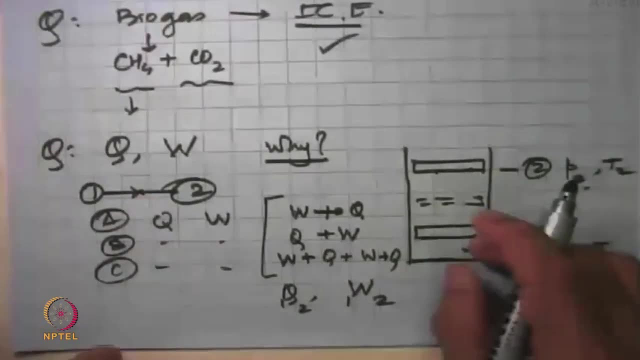 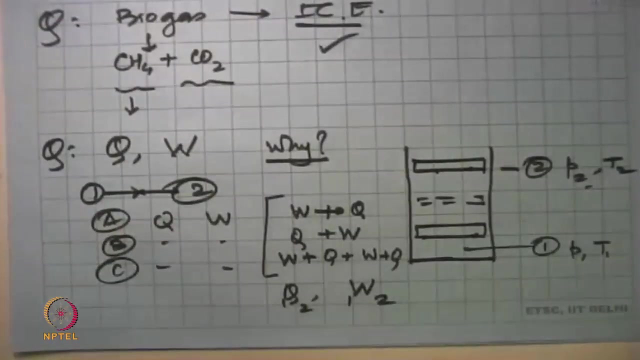 whatever we had asked for, but in each one of these, when we do the calculation, the Q and W for the process- Q 1 2 and W 1 2- these will be different. The exact numbers that will fall on this will come to that when you look at the laws and 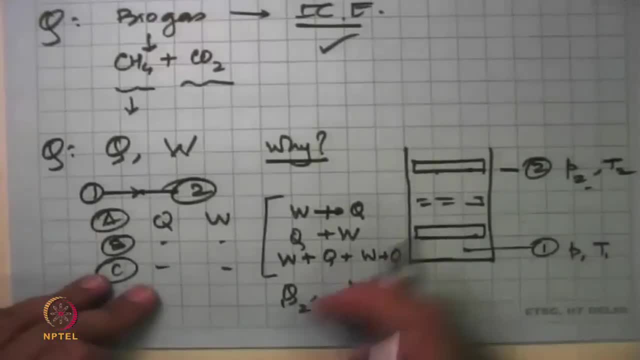 financial properties. when you look at it, then you do a numerical and you will see that Q 1, 2 at part a, where you first heated it and then expand it, or second, when you expand it and then heated it, those heat and the work with those process will be different. ok. 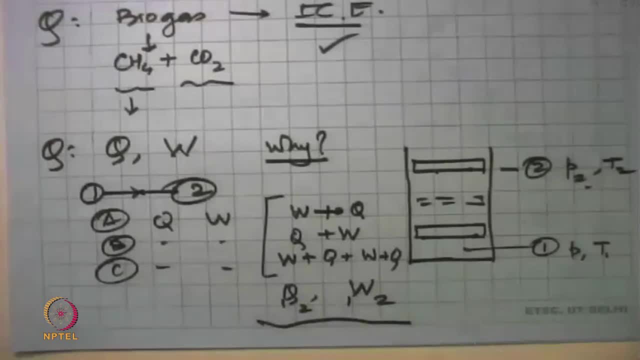 So for now I will leave this example here, But you have the process. So let us see that. But we will come back to it again and again in the next two modules and also in the final module when we solve problem. We will come back to this many times. 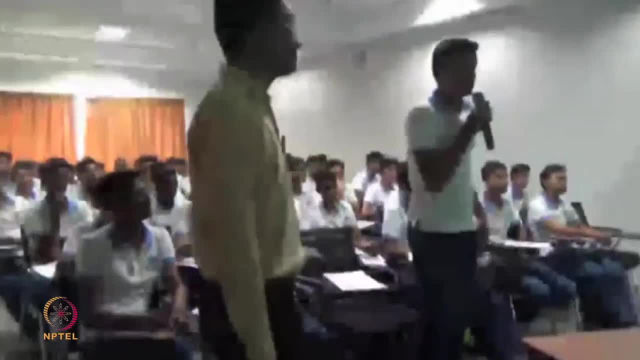 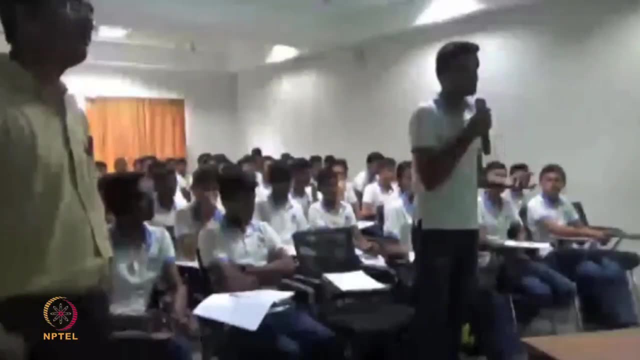 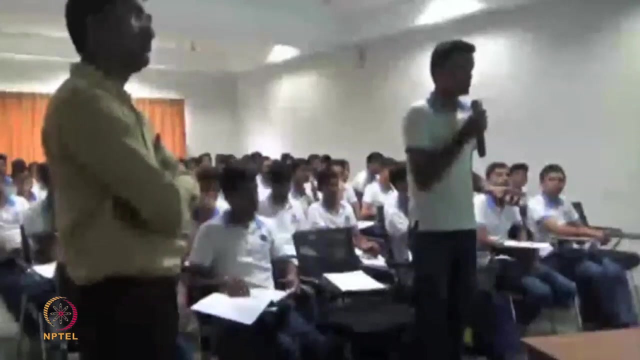 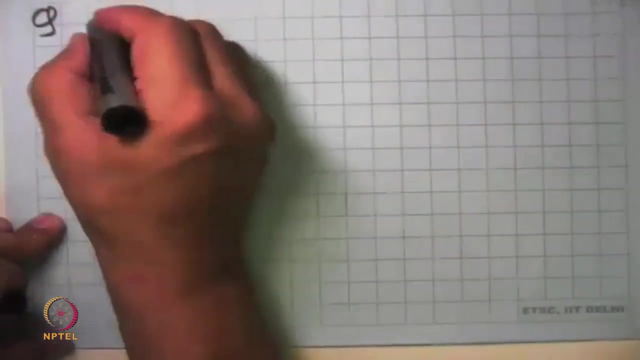 Hello, good afternoon sir. My question is: every reversible process is a quasi-static process, then, but every quasi-static process is not reversible process. why is it so, sir? Ok, This is that we are talking of a process and we are saying- I will not use the word quasi-static. 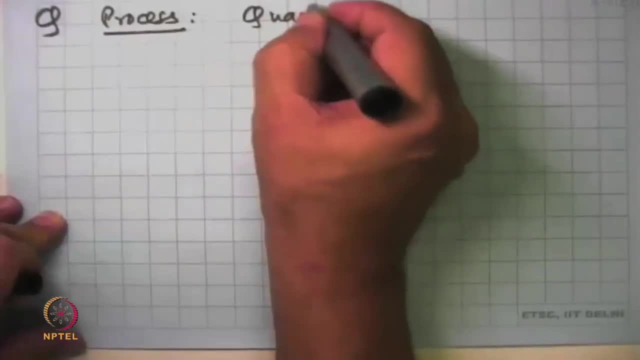 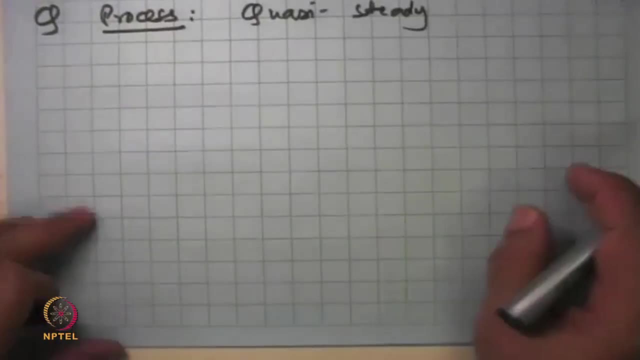 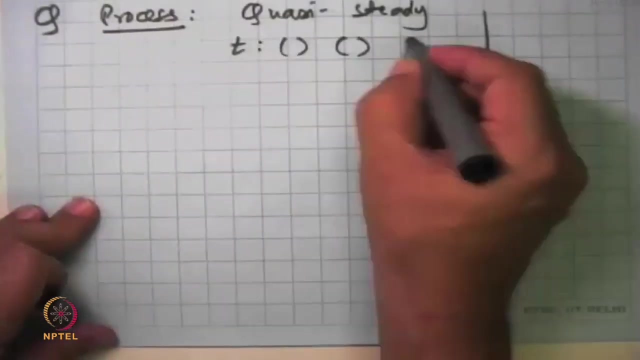 I said the quasi-steady process. In the quasi-steady process, what we are saying is: at any instant of time, we are assuming that the system is in equilibrium. Ok, In between the times, Ok, The system may not be in equilibrium. 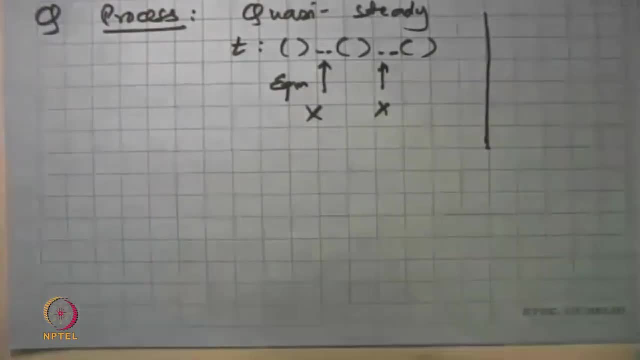 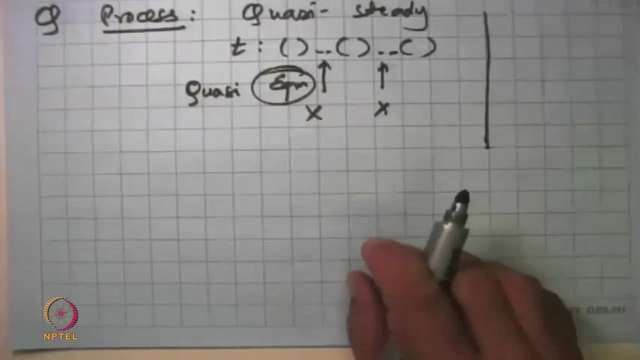 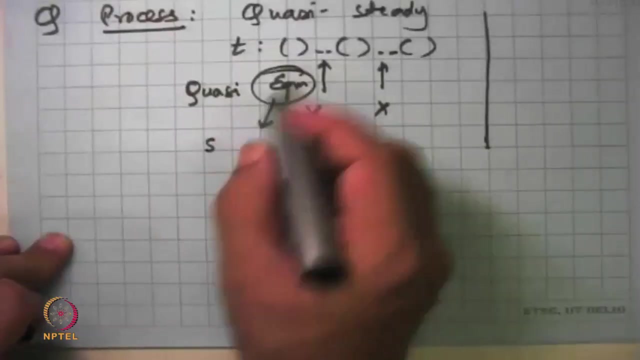 The second thing is, in reality, the system may not be in equilibrium, and this could be in quasi-equilibrium. So that difference is there: that equilibrium is defined only for a state, whereas a process being quasi-steady is for a process which is a change of state. 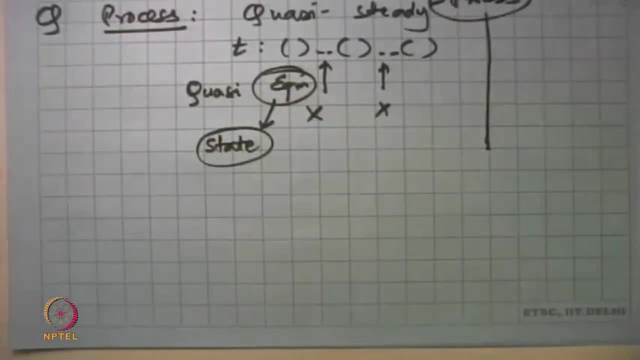 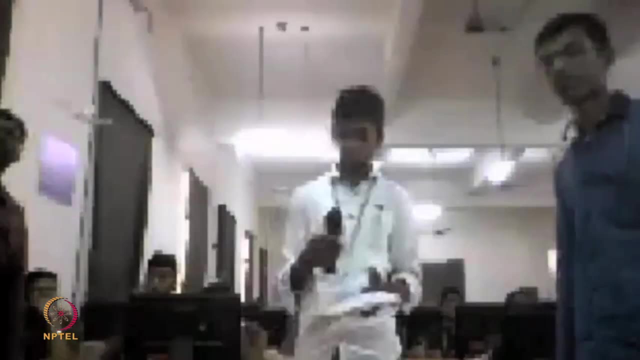 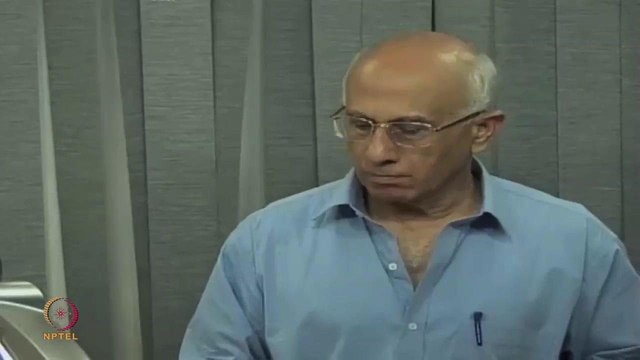 So two are very, very different things. they are not the same. Ok, One last question then. the remaining I will put up on the webinar. Sir, what is the advantage of reversible process? Ok, So the question is: what is advantage of reversible process? 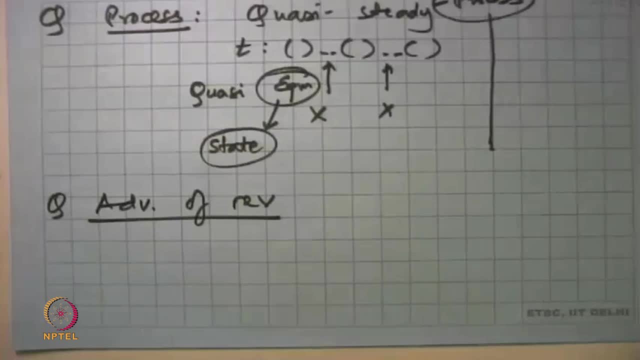 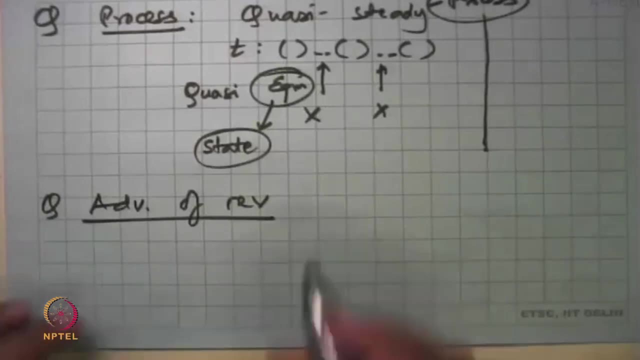 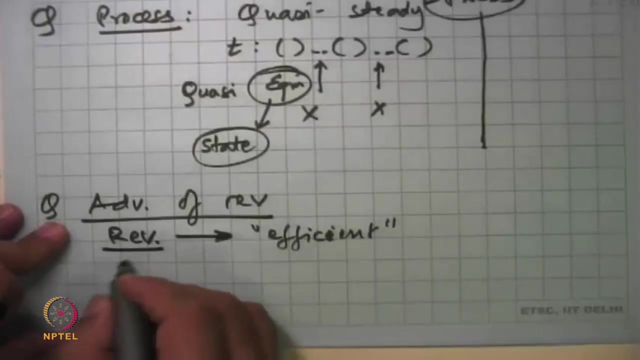 Ok, This is a good question. Ok, Thank you. So, totally, from a definition, the reversible process is something which we will see later on as being the most what we call efficient process possible, And what it does is if you can get reversible, if you have reversible work or reversible. 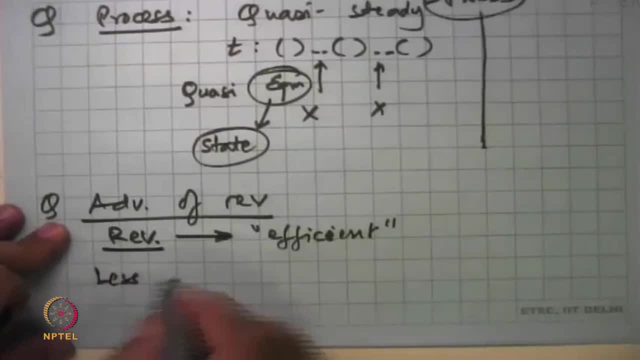 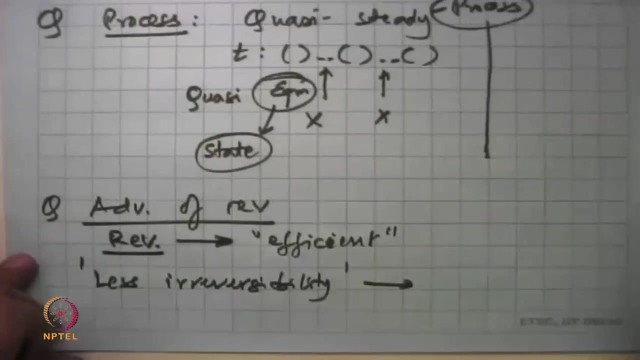 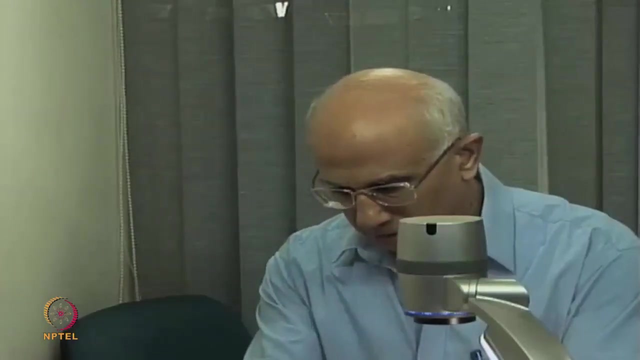 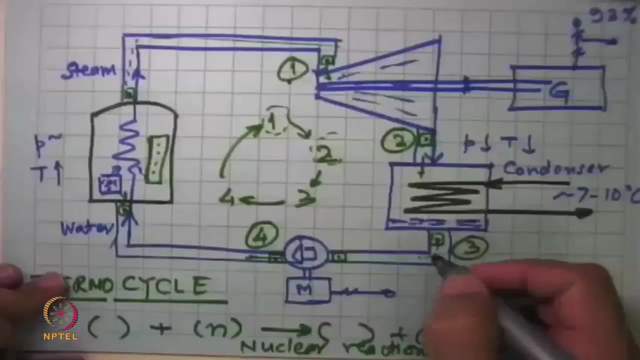 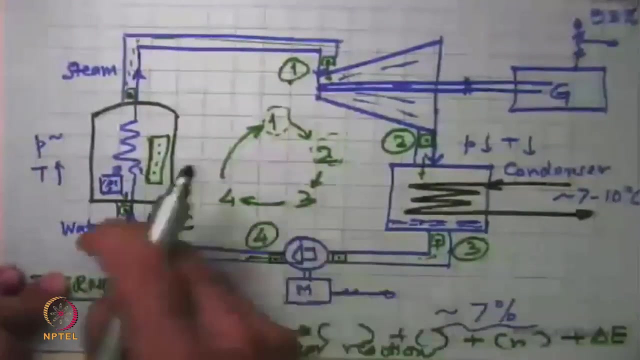 heat transfer. Ok, So the less the quantity, amount of irreversibility, the more is what you can gain as output. Ok, I will go back to the schematic of that nuclear reactor, that system that I have done Here. When we cool water and bring it down to, say, say, 45 degree Celsius, then we heat it in. 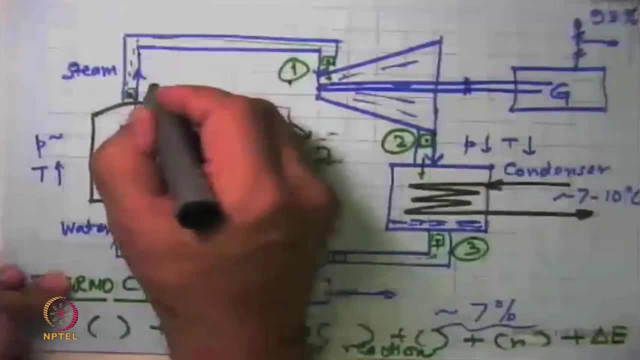 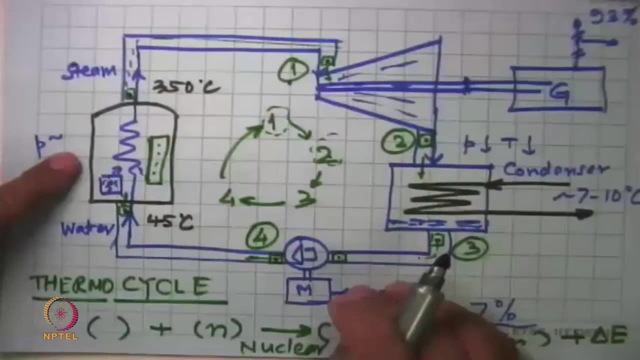 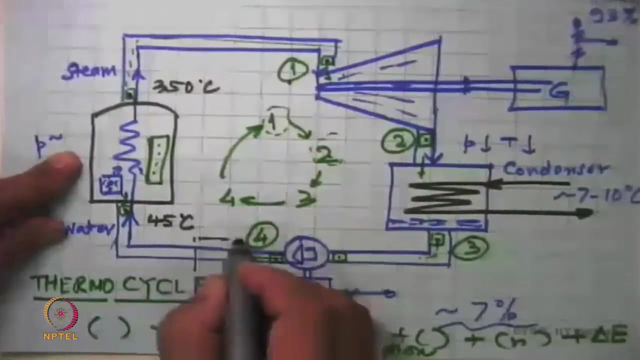 a boiler or a nuclear reactor and bring it to, say, 350 degree Celsius, That means we are using a high temperature source to heat water from 45 to 350.. But if somehow we can heat the water here by using some of this steam or not this steam- 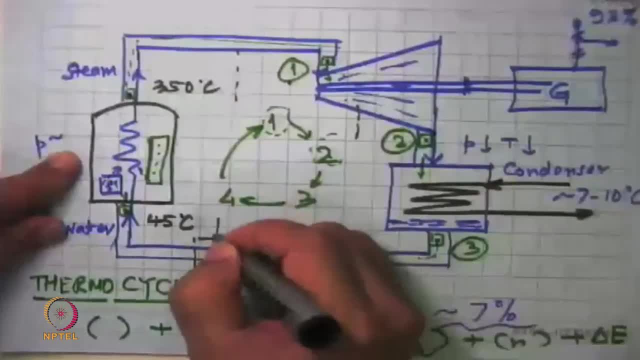 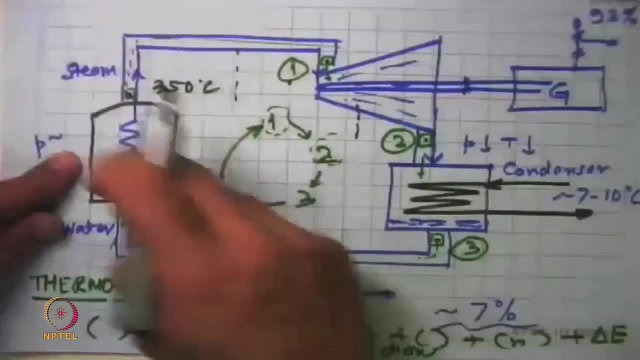 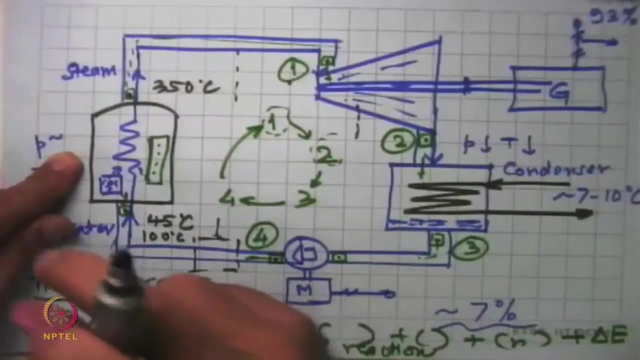 some of the steam from here and raise its temperature to, say, 100 degree Celsius, then the heat transfer in the boiler or in the reactor will now occur over a smaller temperature difference. What that did? It reduced the irreversibility in the heat transfer process. 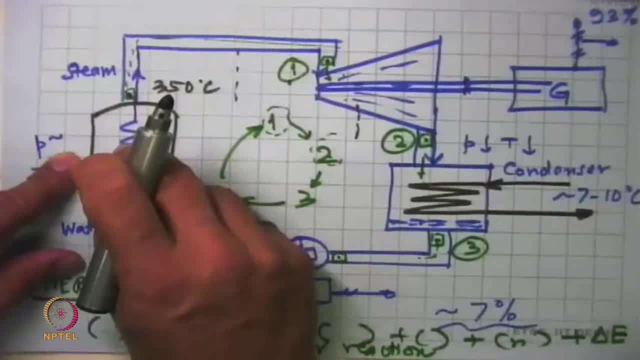 And because of that, it reduced the irreversibility in the heat transfer process And because of that, it reduced the irreversibility in the heat transfer process. Ok, And because of that, the efficiency of this cycle went up, and that is what we try to do. 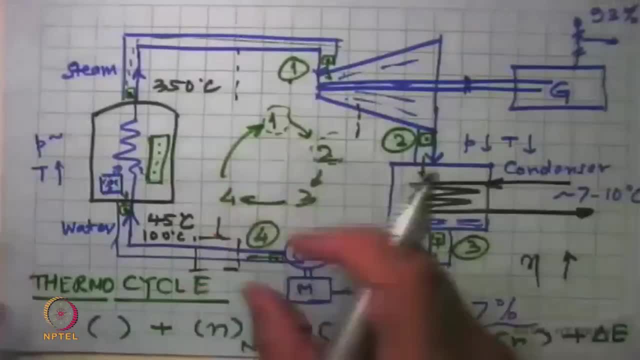 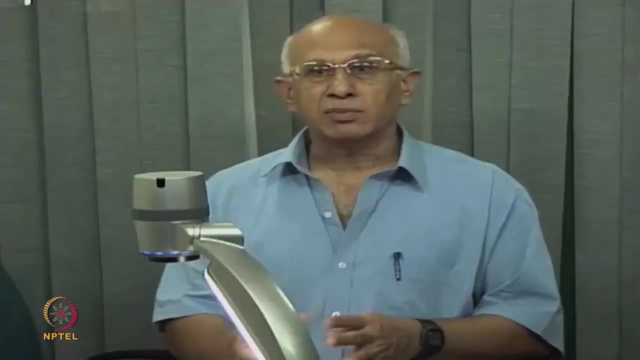 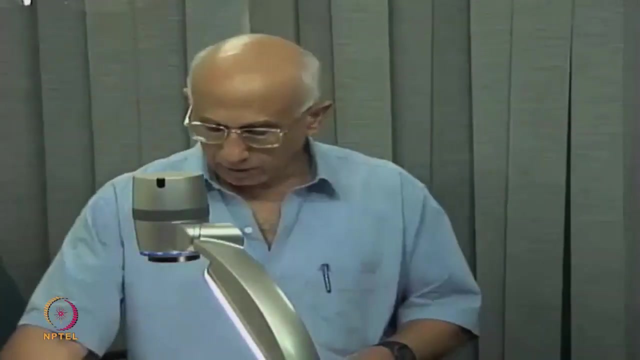 in many of the devices is that if there is heat transfer taking place, we try to reduce the temperature as much as possible. That way the system may get more complicated, system may get bigger, but that becomes the most efficient thermodynamic system. In later on, when we look at ah cycles we will find that the reversible cycle is the most. 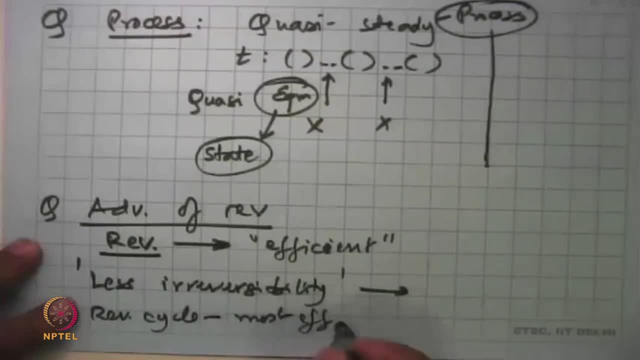 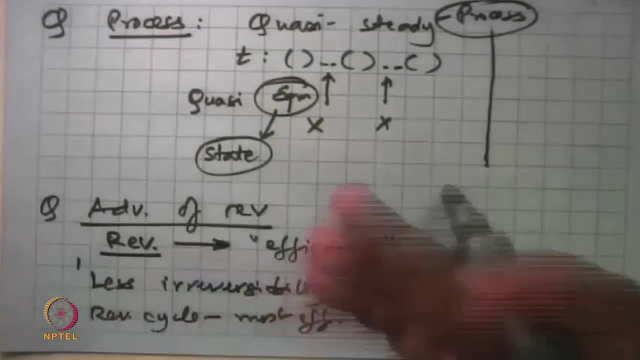 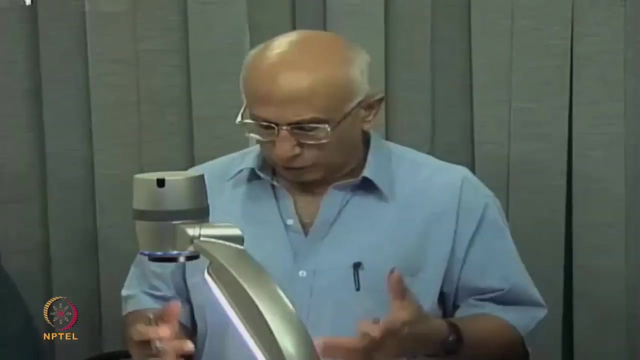 efficient cycle cycle, say, from converting heat to work, And we will see that to get it reversible, everything has to be very slow. differences have to be very small. friction does not have to be there, which it should always be there. It is extremely slow and very, very difficult to make and practically 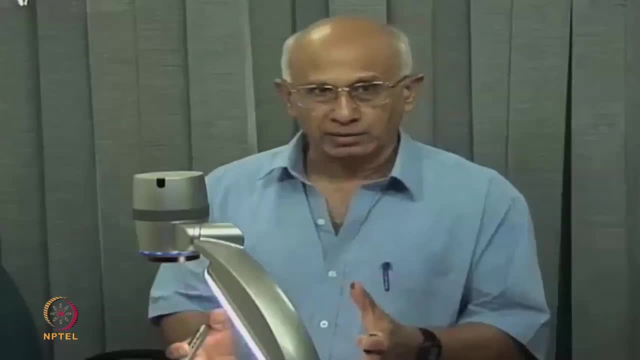 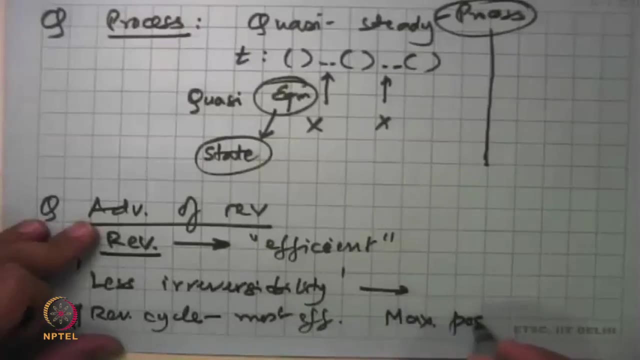 impossible In reality. you want everything fast and quick, but this gives us a benchmark of what is the sort of the maximum possible efficiency, if I want to call it efficiency, or the work, or the heat that I can get from the process. That is why reversible process. 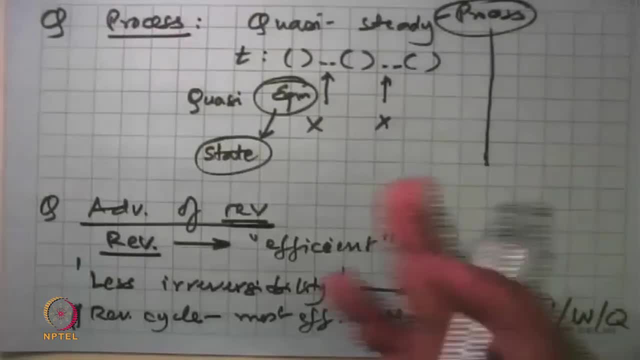 is a concept which tells us what the best possible thing you can achieve and in reality we do everything to get to that process, So that that is the only advantage that we have in this concept. We will come back to this again when in all.